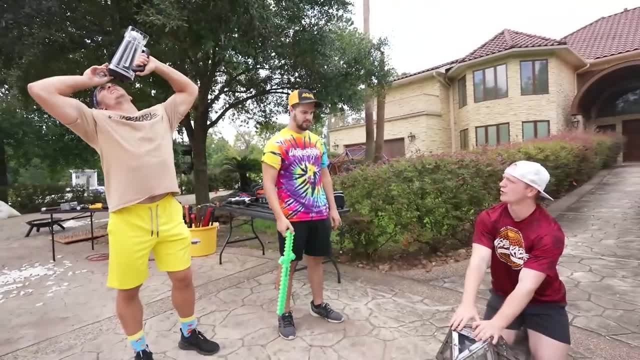 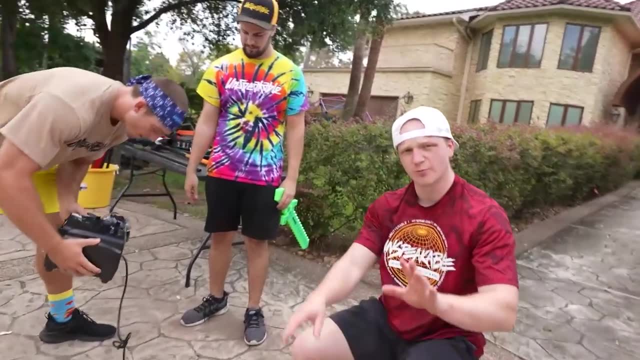 How are we gonna break into this thing? What's gonna be our first weapon of choice, James? Oh sorry, blender. make it into a smoothie. We're gonna blend it. We're gonna blend it. That can be in a blender. what we're gonna do here with this amazing. 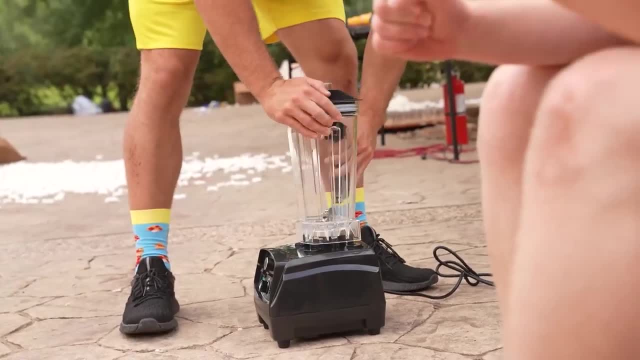 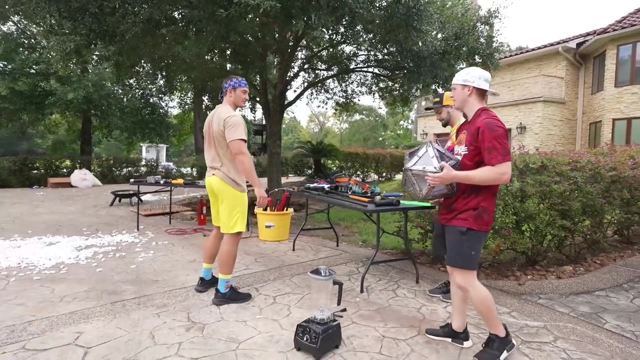 Unbreakable is: we're gonna start off with a simple weapon. that weapon is going to get stronger and stronger and at the end of the video We will break into this thing. I don't care if it takes two days or three months. Alright, just drop it. Let me go get an extension cord. Okay, go get the cord. I'm gonna drop it on this thing, Wait. 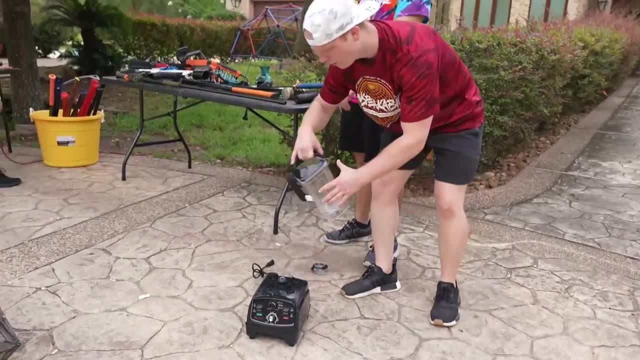 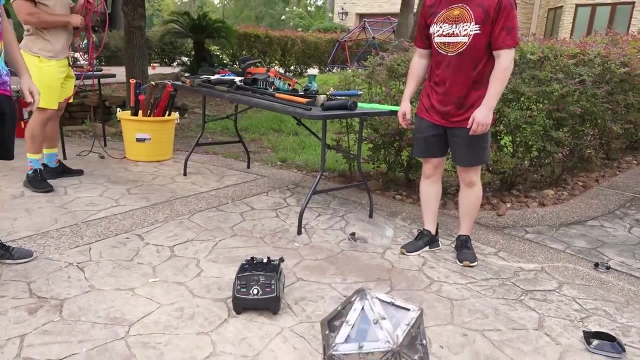 We're supposed to plug it in first. Oh, Open the lid. Ah, there we go. You're gonna plug it in. Yeah, I'm getting the card. It bounced off the blender for some reason. I got a court. gets gonna fit. no, fit here. 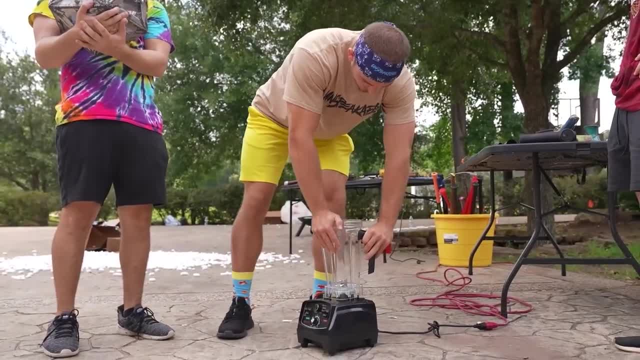 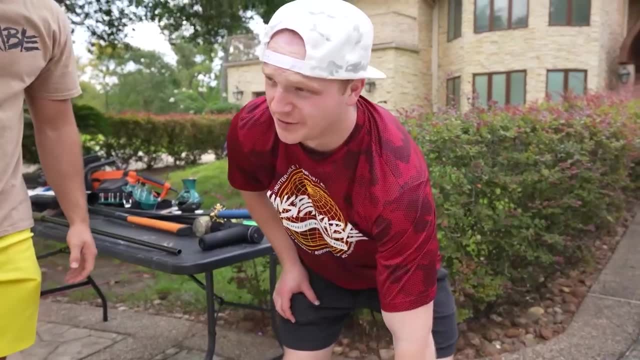 James, you know how to make stuff fit that. a bang, but a boom. this thing smells like my shoe. It kind of doesn't smells bad For our next item, I think if we'd be really nice to the cube and, just, you know, make it relax. 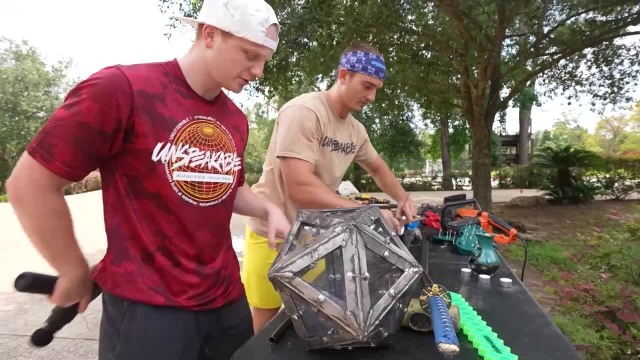 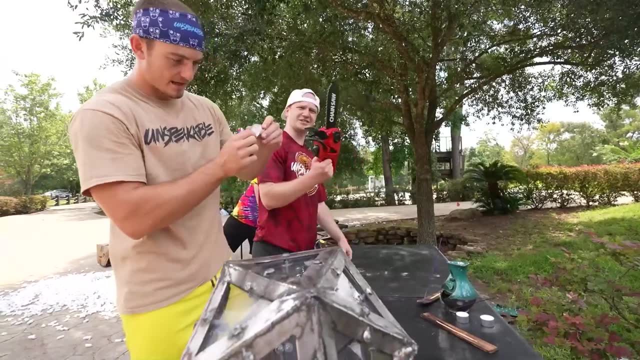 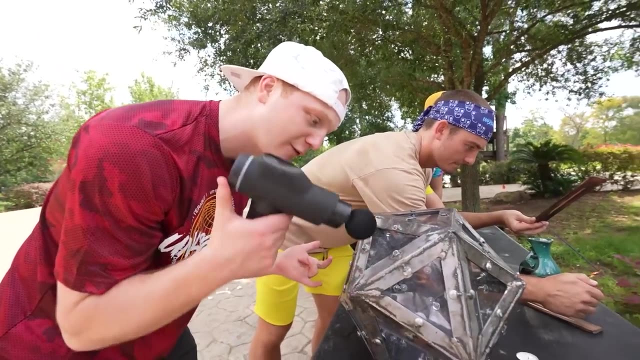 I think it might just open up for us. We get some can, Oh yeah, get some candles? Yeah, All these weapons are scary, bro. One of these: spike shoes, chainsaw. that's nice relax, but it's gonna be okay. You're about to enter a nice massage. This massage is a hundred fifty dollars an hour. It's very fancy. 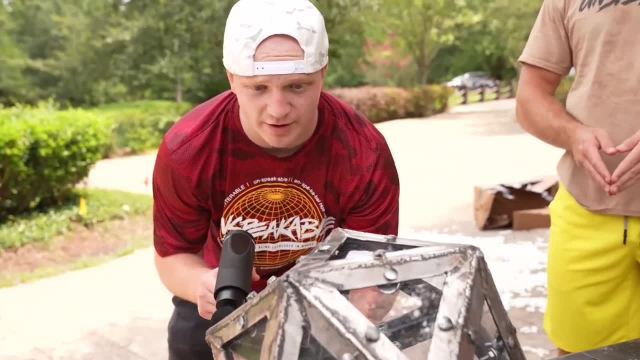 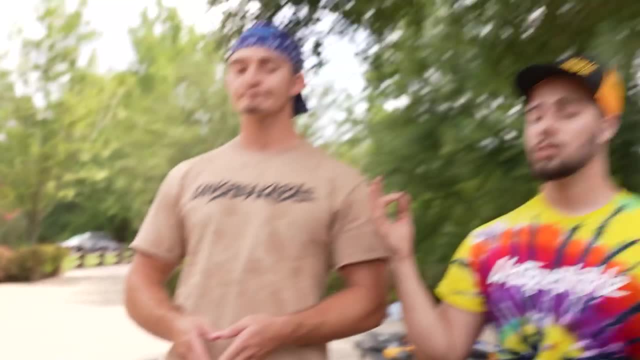 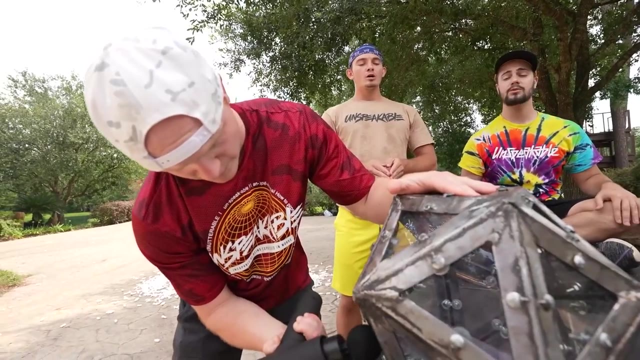 Excuse me, sir, Are you ready for your massage? Okay, just go ahead and close your eyes and listen to me breathe in. If there's too much pressure, just let me know, I can lighten up. And, through the nose, out through the mouth, deep, slow breath. 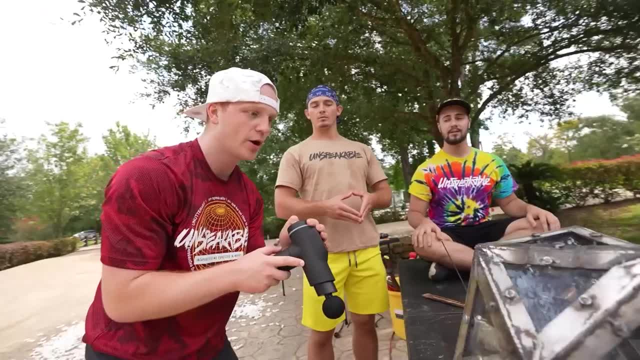 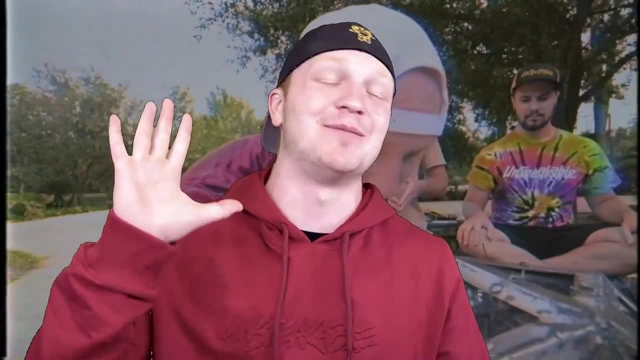 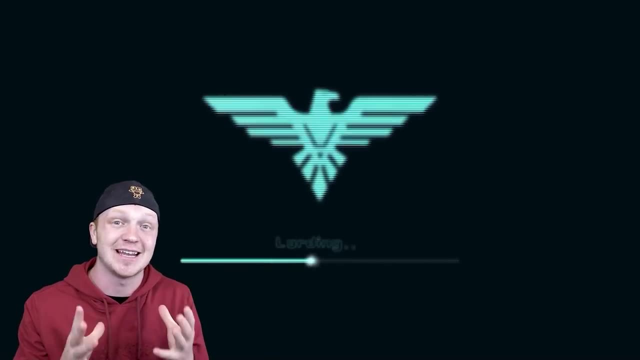 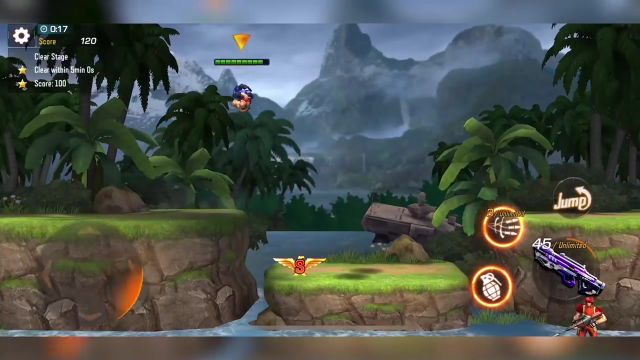 And through the nose, out through the mouth, You'll be ready in a moment, Actually working. he's opening up. look at this: with the vibration that screw is coming off. I'm sorry, I didn't mean to pause today's video. I know you're really enjoying it and I promise it's absolutely epic. 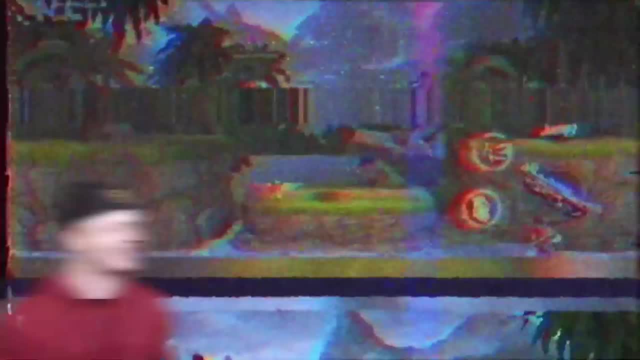 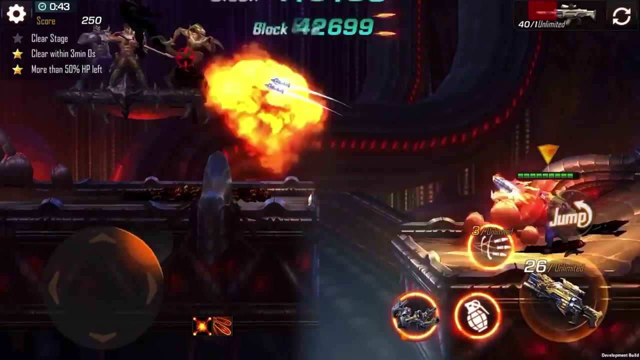 So continue watching. I came here because I want to thank today's sponsor, Contra return. 187?. That's older than me by like 10 years. Contra Returns is now bringing its epic action experience to mobile game rules around the world, Available on iOS and Android. Contra Returns has 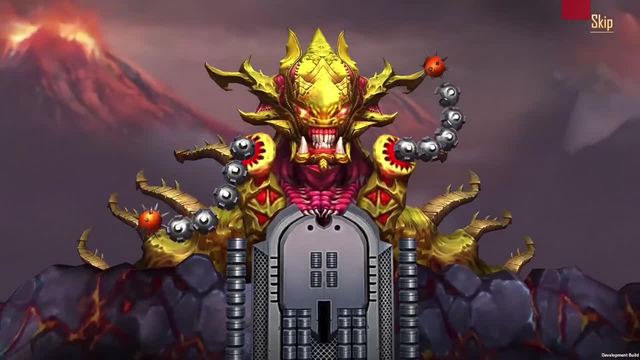 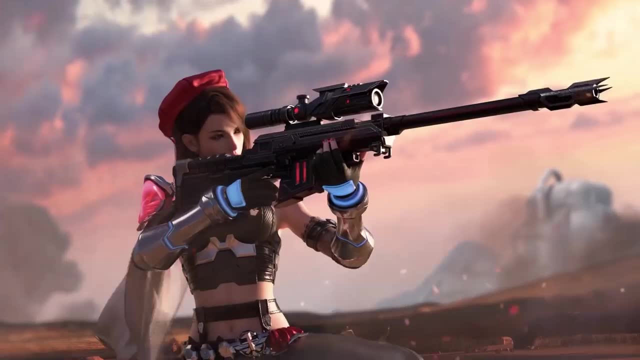 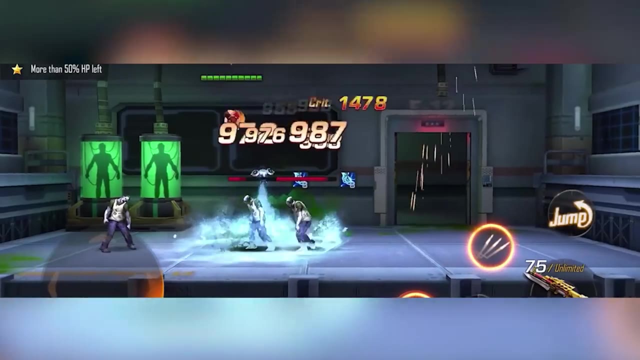 over 200 plus levels of intense actions, as players can engage in single-player run-and-gun game experience or go head-to-head in real-time 1v1 or 3v3 multiplayer action. You can choose from more than 10 different heroes that you can upgrade and enhance with unlockable skills. 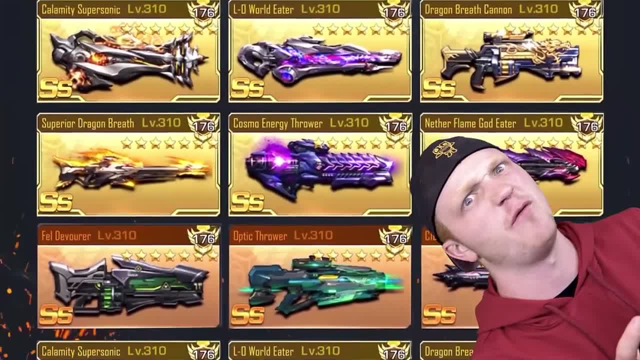 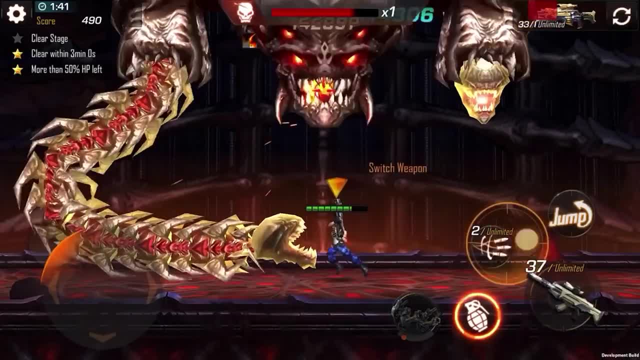 and pair them up with massive arsenals of weapons. Contra Returns is an awesome mobile take on a beloved 80s classic that you can now play on your mobile phone. Download the game and play it for free from the App Store or Google Play Store. Guys, there's a link at the top of. 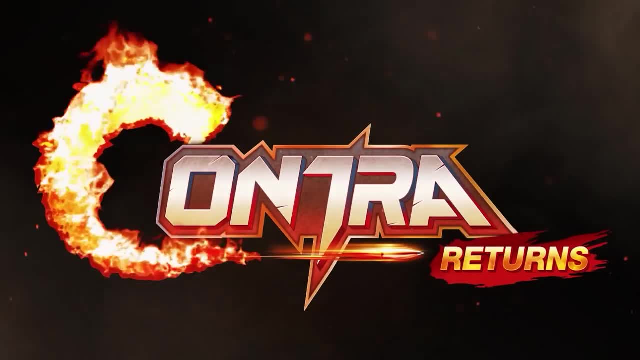 the description. Thank you, Contra Returns, for sponsoring today's video, and let's get back to the action. Oh boy is it messy. If I can get all those screws off, this will come off. Keep going, it's working. 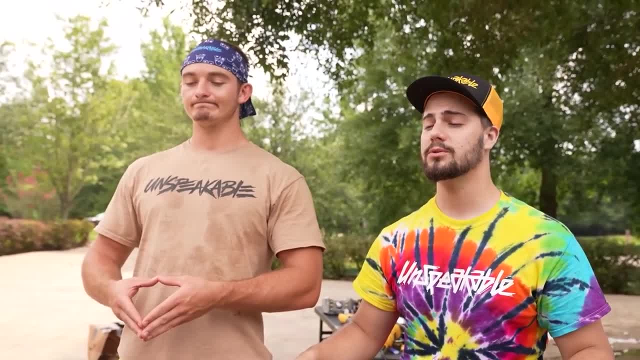 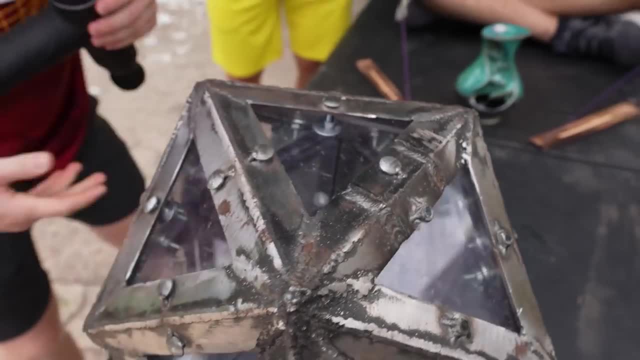 It's working. A nice slow engine through your nostrils and then out the mouth. Clear your mind, Think of a happy place. Oh, it's working. Oh, look at that, It's opening up to us. Yo, I didn't. 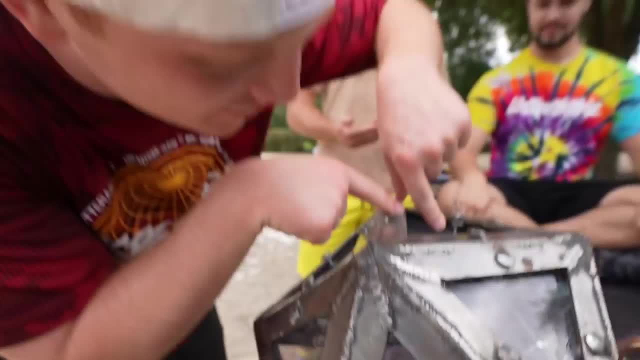 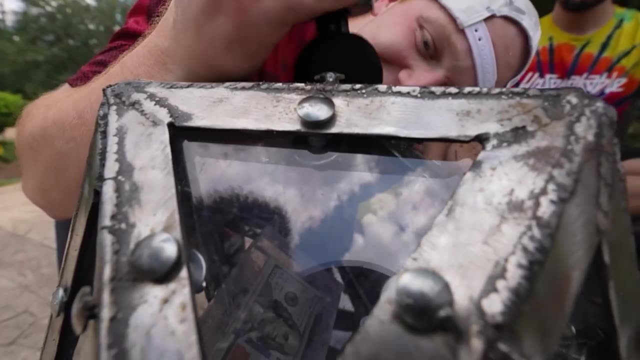 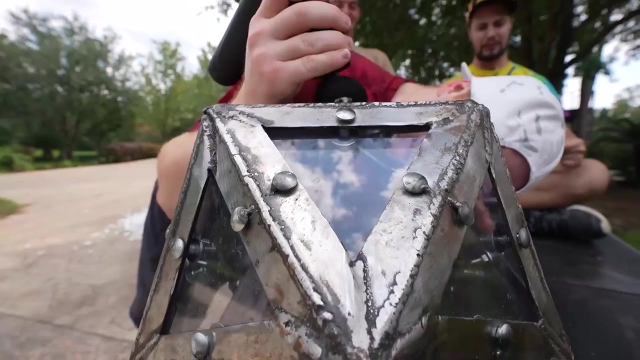 think that was actually working. Of course it's working. I told you: Look at you, see the screw right there. I completely took off that screw. You just got to relax, buddy, Just open up. We're going to try a couple more right here. 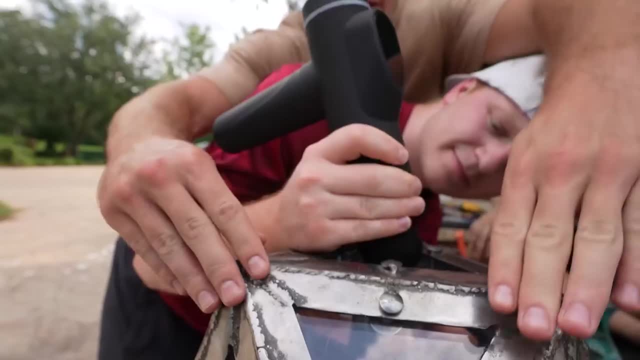 Okay, stop, stop, It's not working. No, it is, it is, it is. Yeah, give it a massage. You like that little bath. Smell, smell, smell, smell, Smell the divine, Let it relax. Look, I got the one screw. 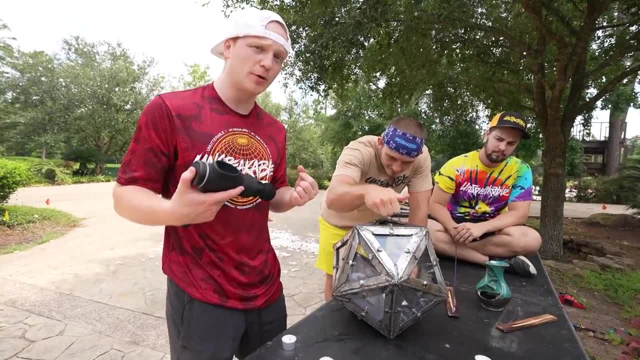 off. It is opening up a little bit. There's two screws that are halfway almost off. What if I check them off a little bit? Oh, that's why. Yeah, I see The nuts are hitting. Oh You sneaky. 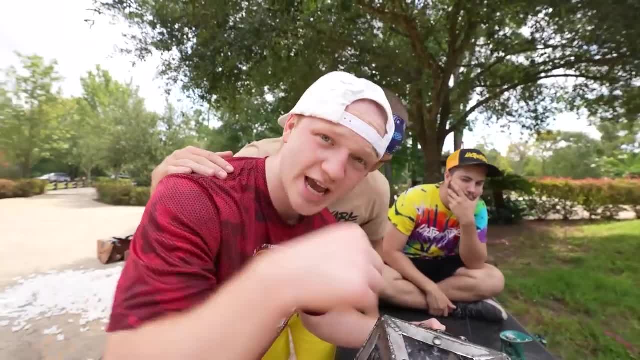 sneaky boy, All right. so what's happening here is the screws are actually hitting each other, so it's allowing the nuts to not fall off. Otherwise, the meditation vibration technique wouldn't have worked on you. It did work on you, It didn't work on you. It didn't work on you, It didn't. 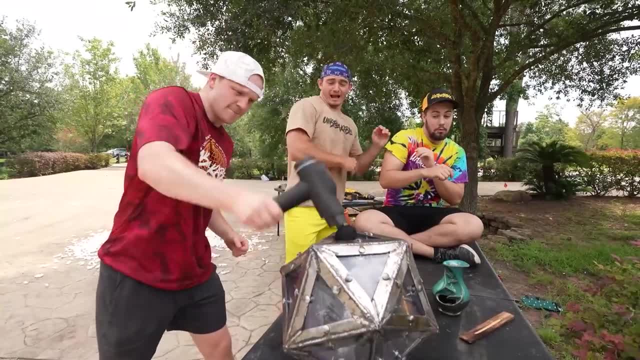 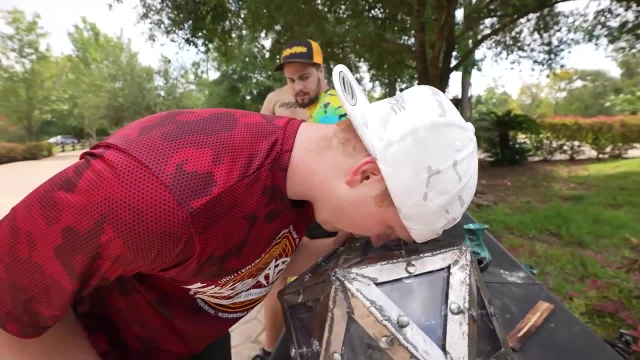 work on one screw. Forget it, boys, It's not working. Oh, Oh, Hey, hey, hey, Whoa, Oh Wait, is that from the gun or the Good question It has opened? Yes, you are relaxed. Are you ready? 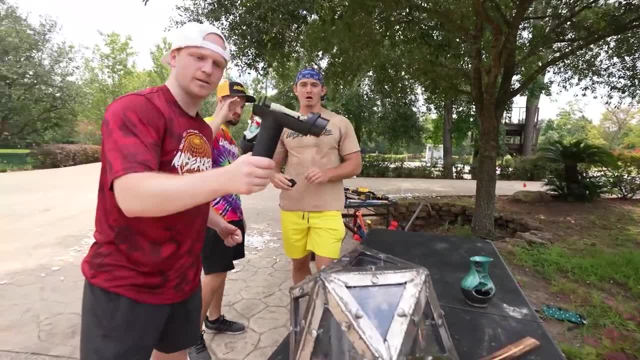 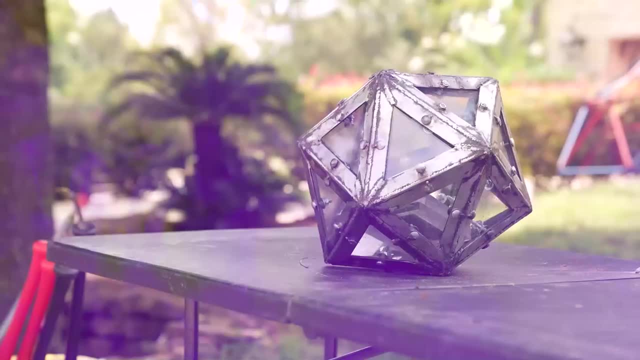 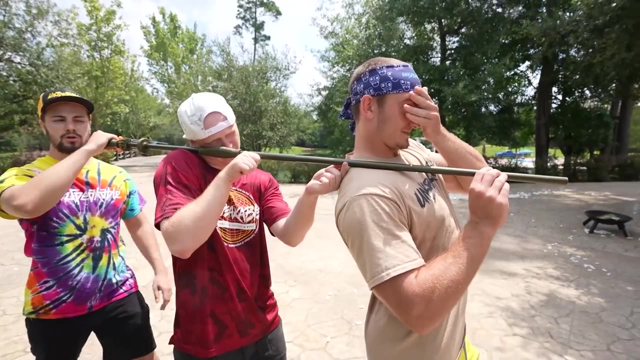 for your next treatment: Flip. Well, boys, our massage business is out of business because this thing's broken. All right, James, just aim at the cue. Ready boys? Yeah, we're ready, I'm ready. All right, Is it aimed? I think so. I think it's good. All right, full power. Move your finger a. 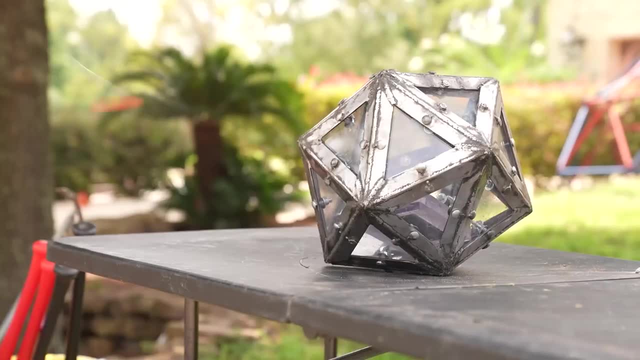 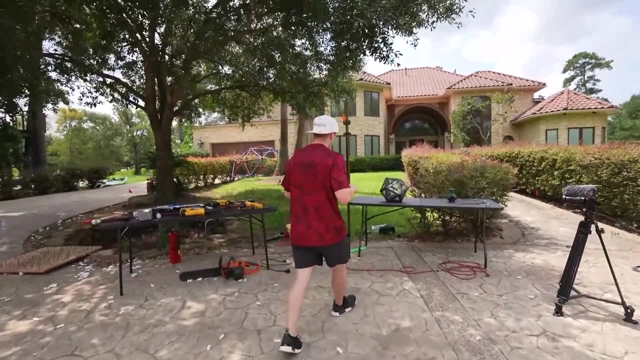 off The dirt, came all the way back. I was scared for my life. What Did it hit? metal or plastic, or one of the glass stuff? I think it hit the plastic. Oh, we do have an indent Mark. Look at that right. 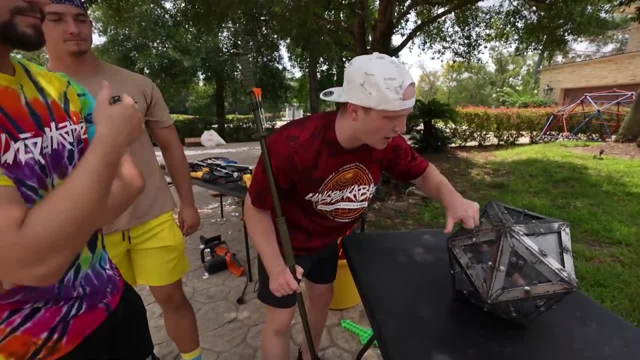 there. Oh yeah, A very, very tiny indent. By the way, guys, this is not glass, Otherwise it would be super easy to break through this. What kind of material is this? I don't even know: Polycarbonate. 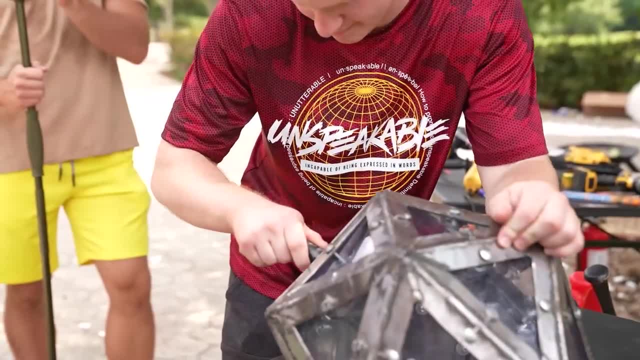 Polycarbonate, Polycarbonate. So this is a glass breaker so I can show up. It doesn't do anything. You know, maybe that one's broken. I think it's for like a car. Oh, maybe you're using it backwards. Try the other side. 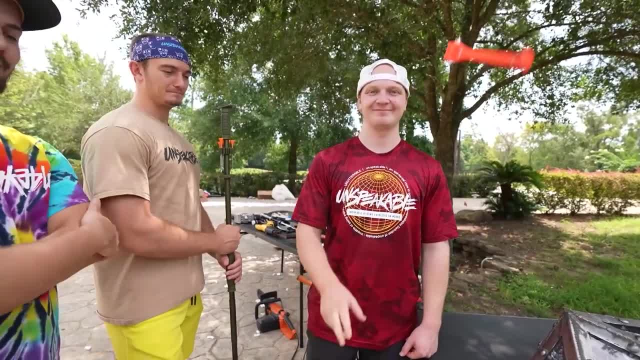 That was loud. As you can see, Boy, it's hot, It's not glass. No, Any of y'all got a chainsaw by any chance. I think I got a little one Chainsaw trap. All right, yo, this is getting. 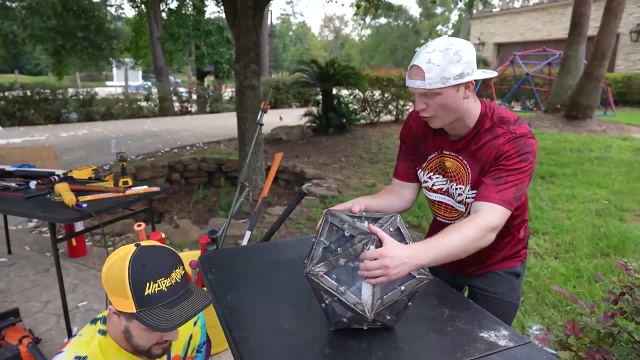 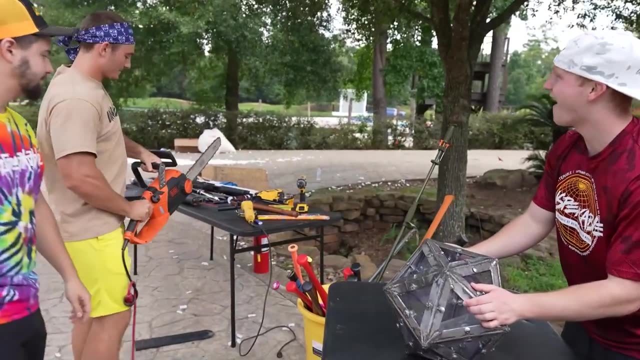 really loose right here. If you could come in with a chainsaw and cut it right here, go for it, Bro. bro, stop, Stop. Sorry, that's the wrong one. He's got the real one. Oh, there we go, Ah. 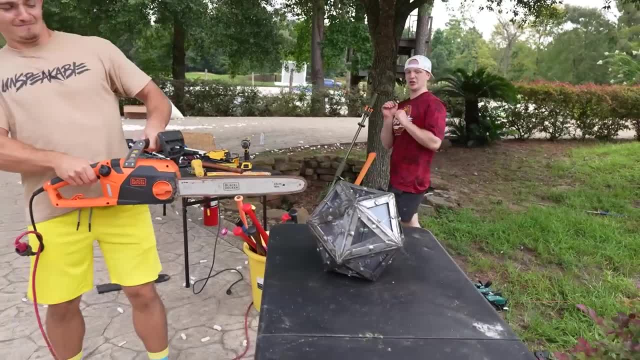 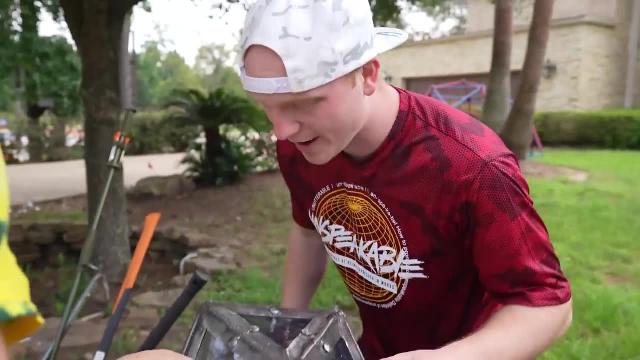 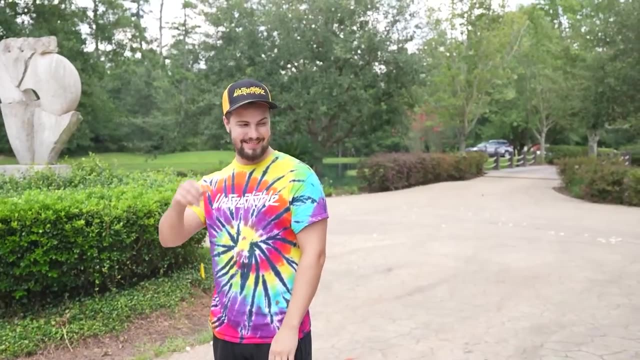 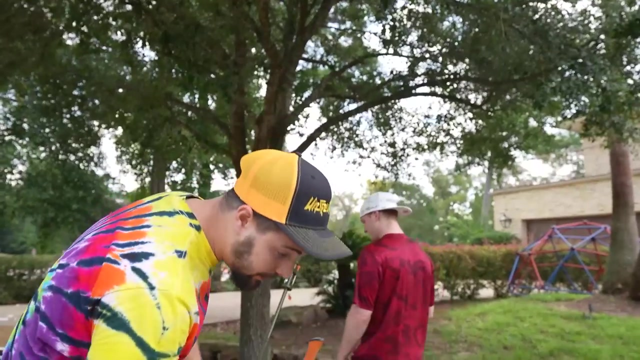 there we go. All right, so we need to cut this triangle. Is it working? Analysis- Yo, it's not bad. Yeah, yeah, Keep going. Look at that. You probably got like a fingernail. Oh, it's smoking. Kowalski analysis Damage. Wow, that's thicker than I. 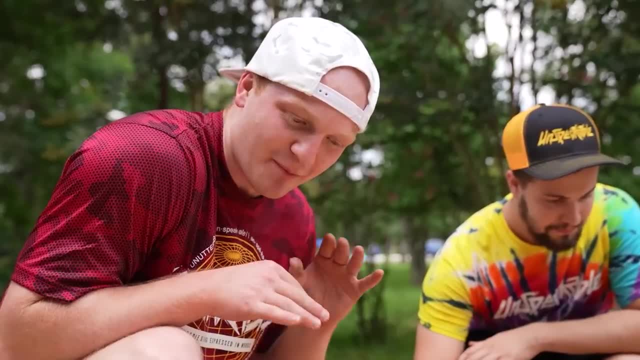 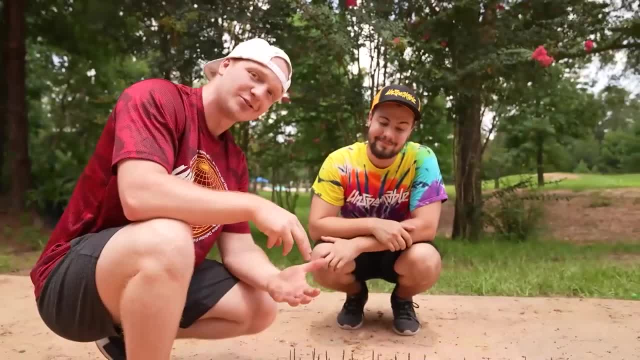 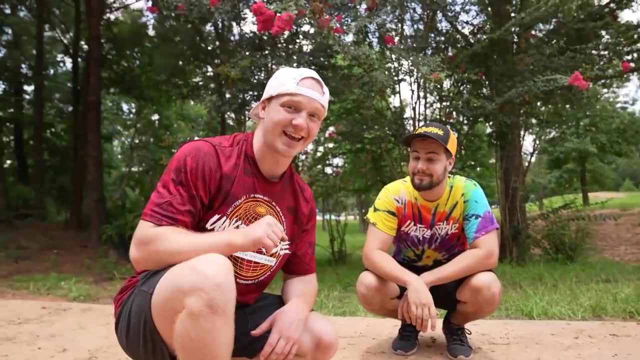 cube on this and we're gonna see if the nails penetrate it and hopefully break most of the plexi quality carbon plastic blast, whatever you call it prediction. i don't think anything's gonna happen. i think it's gonna break the nails. okay, if that is the case, we have more weapons up there to. 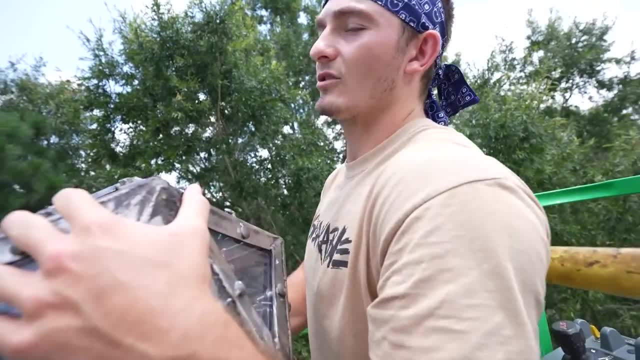 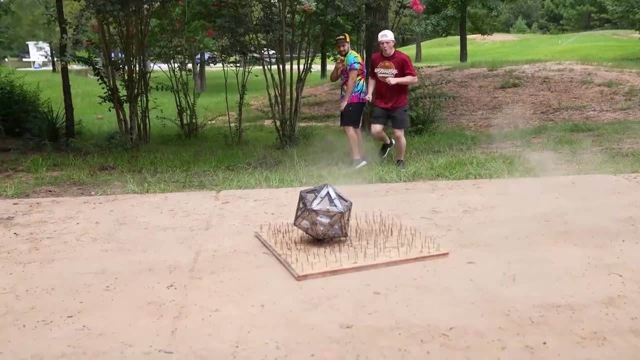 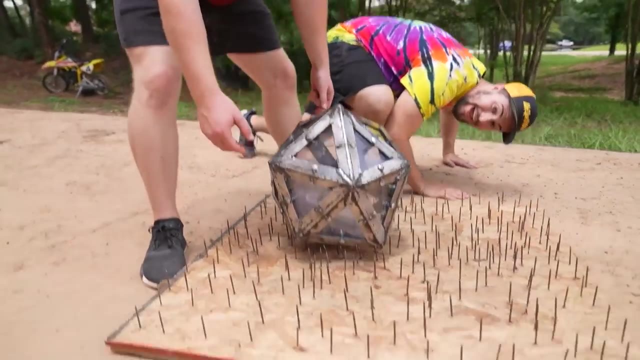 drop on it. all right, let's go. this is like a trapezoid right angle, obtuse triangle prison ball. all right, you ready? yeah, three, two, one, here it goes. oh, oh, i think it works. oh, it's stuck to the plate. hold on, lift it up. oh, bro, i can't lift it up. it's stuck. oh, yeah, it is. oh, here i can lift. 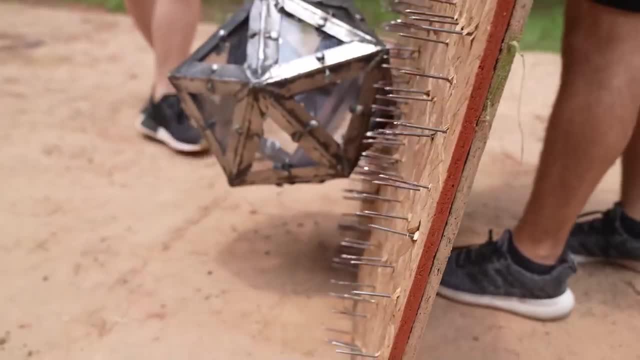 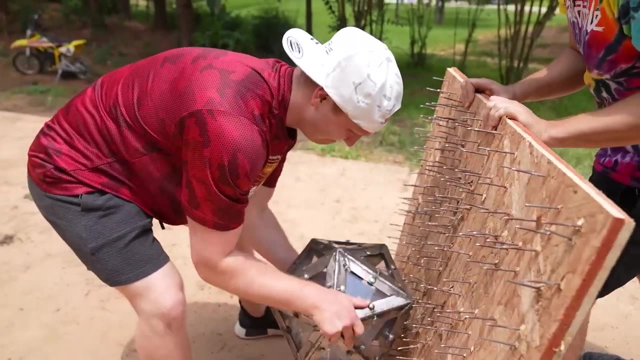 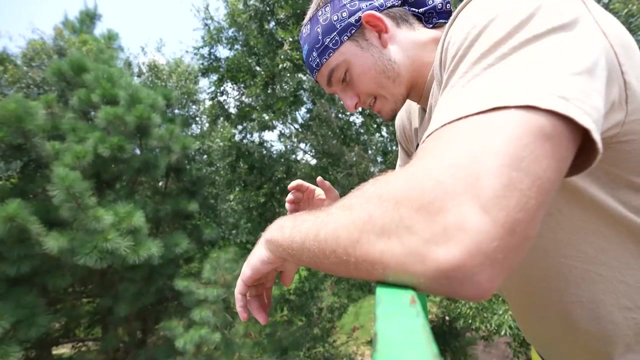 up the board. hold on, just lift up the board, look at it. oh, it's stuck, right, it's stuck. there is a couple nails that are straight in the board. i can't. okay, oh, look at that, we pulled the nail all the way through the board. okay, so damage analysis: plastic has broken. we do have a nail. 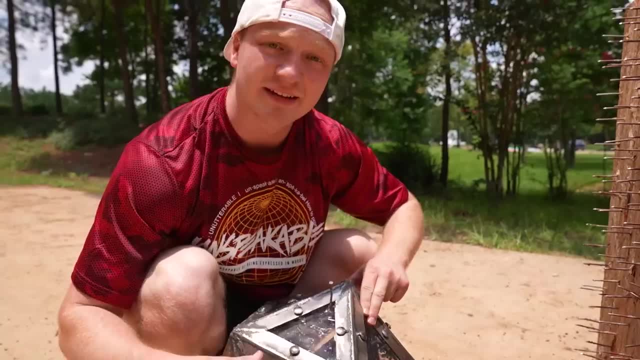 that is pretty deep in here. look at that. that nail made it all the way through to the other side. that did not work. it did not work, make it through. we did not bust open the cube. so now what if we drop a bowling ball on it? yes, 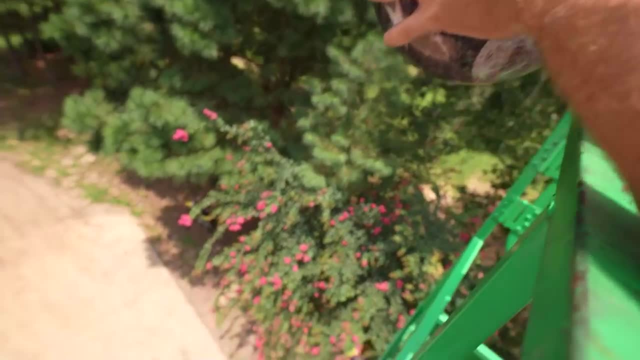 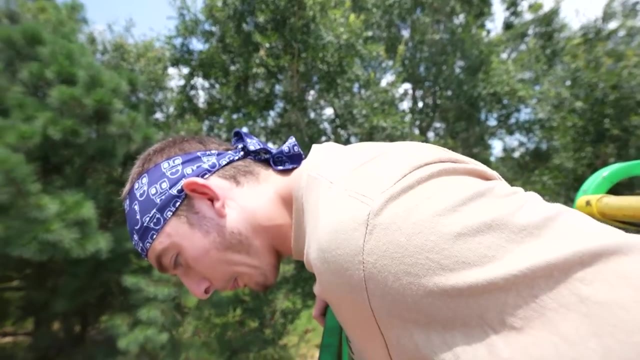 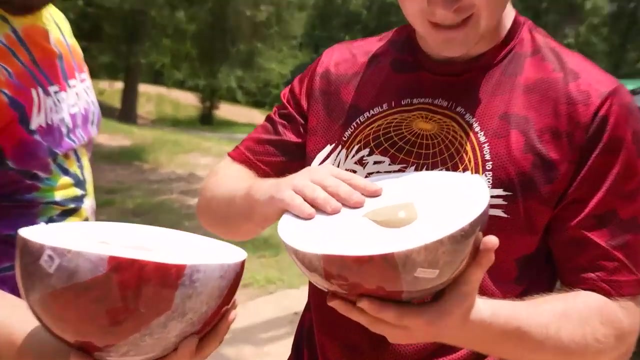 yes, you guys ever see me bowl. i'm a pro ready when you are all right, ready? oh, no way. no, what, bruh? i've never seen that happen. yo look how clean the cut is. what i've never even seen the inside of a bowling ball. what is that? is that a coconut? look at how clean that cut is this ball. 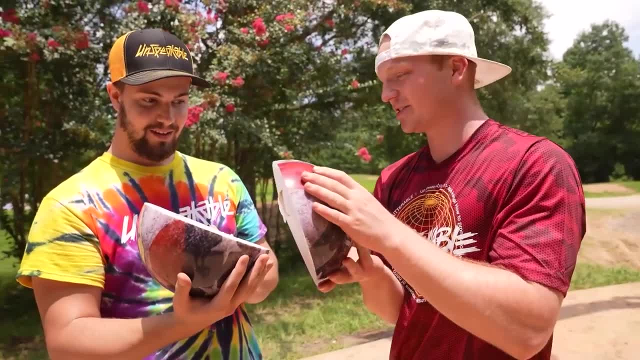 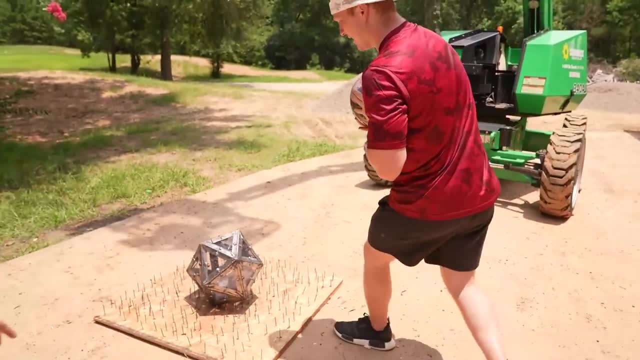 was not previously cut. this is a brand new one. bowling ball- oh my gosh, just put it back together. we got to put this in a box and hanging up on the wall, so this is like where it impacted. it looks like it impacted the top of the cube right here. 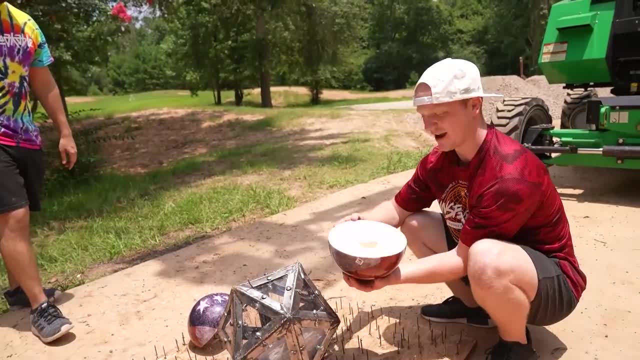 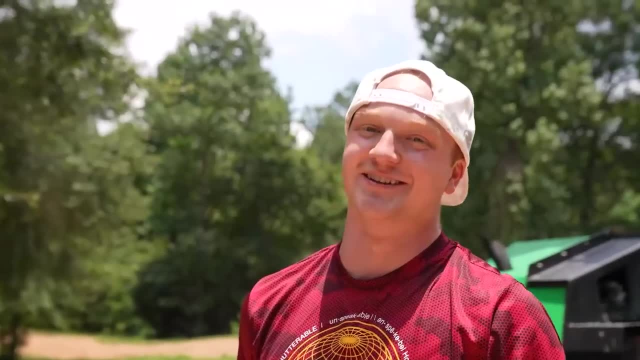 or somewhere around here and literally just landed on it and split it right in half. oh my gosh. wow, that was the last thing i would have expected. i was not expecting that, okay. well, now we got the cube versus the tungsten cube. you guys know the time we're going to drop it on here, if that thing. 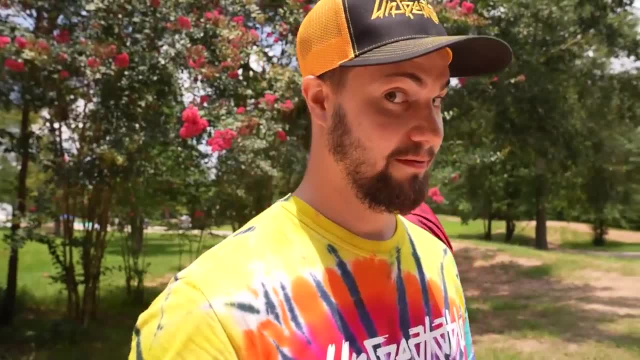 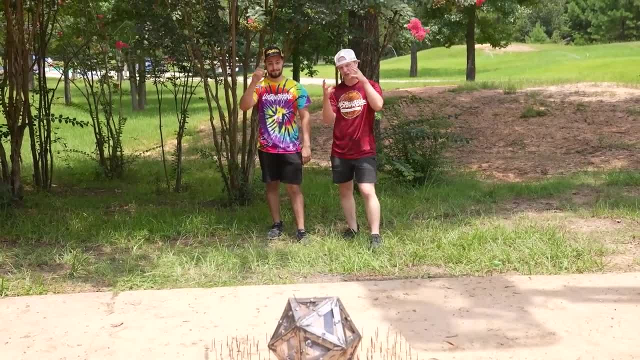 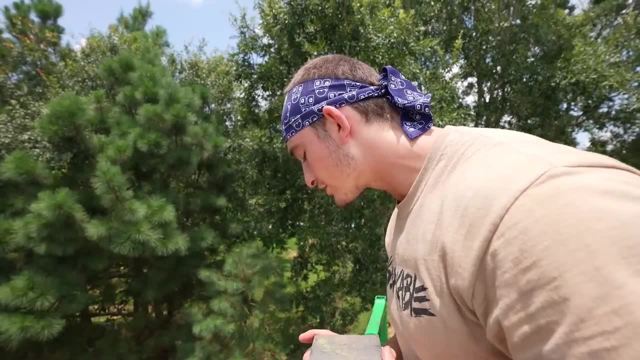 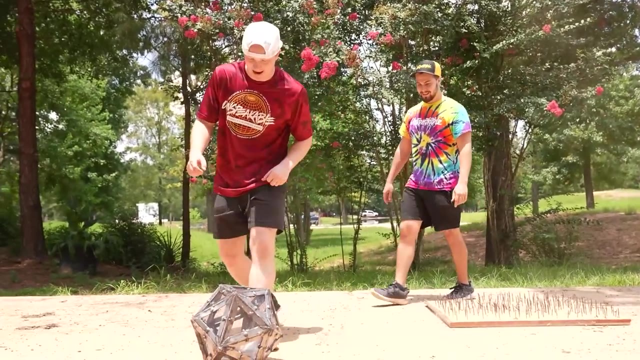 Now it's time for the tungsten cube. that's almost 45 pounds of a solid tungsten steel being dropped on that. it's basically as heavy as an anvil. all right, i'm gonna give a countdown to this one, because it might hurt someone. three, two, one drop. oh oh, bruh. okay, so we have direct impact on the cube, i'm not sure where. 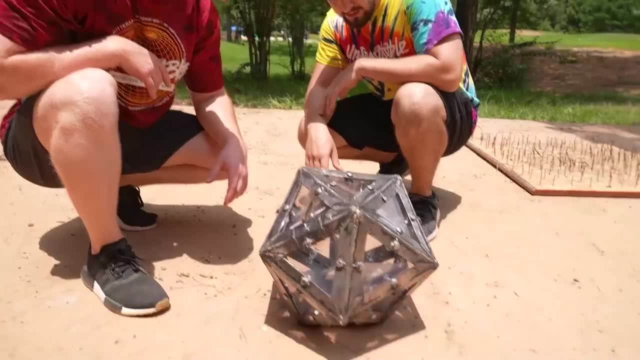 it hit. i don't really see it had to be a piece of metal it hit. i don't really see any damage. oh, right here, right here. oh yeah, it's into it right here. check that out. you can see a huge dent right there. you can see that line. that's right there. you can see that line. that's right there. you can see that line. that's right there. 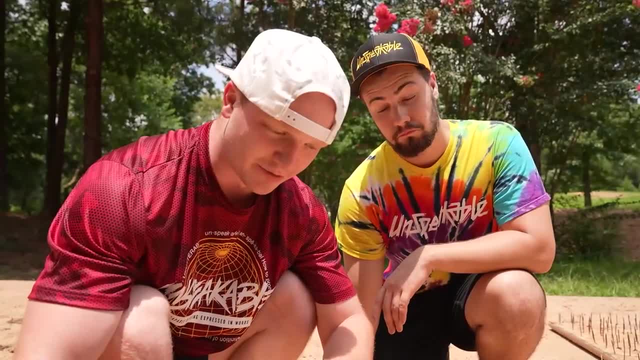 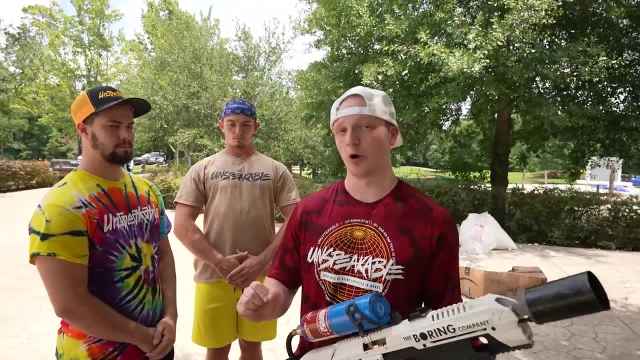 line. that's where the corner of the feet hit. so we have a large dent, but nothing is really broken on it. i think we need a bigger weapon. yeah, all right now. our theory is to burn. you see, okay, everything in the world melts at a certain point. there's a melting point for everything you. 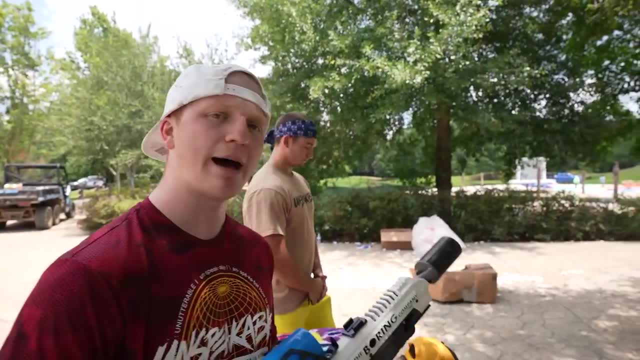 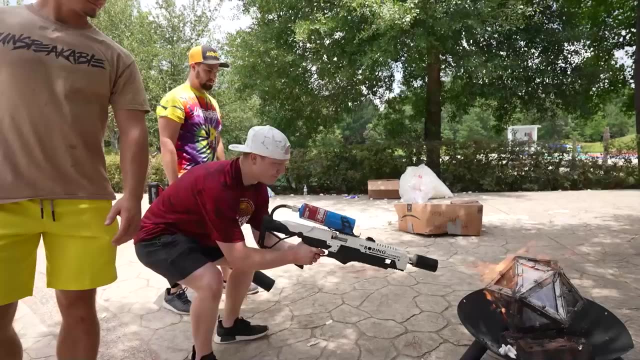 can steal titanium tungsten. anything melts. so if we can get this bad boy hot enough, you completely melt. it would also melt the money inside. so let's see if it works. oh, that's hot. yeah, baby burn. get the logs going, hit the logs, yeah, all right. so we're just gonna. let's see if it works. 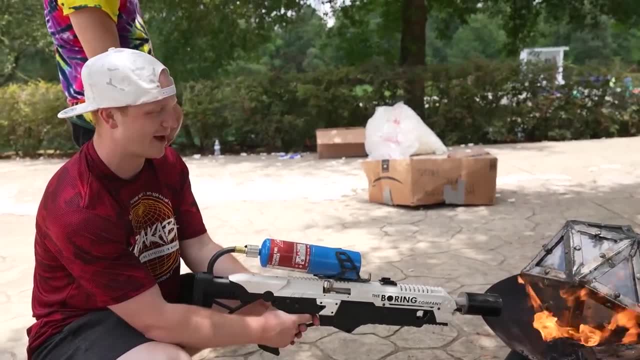 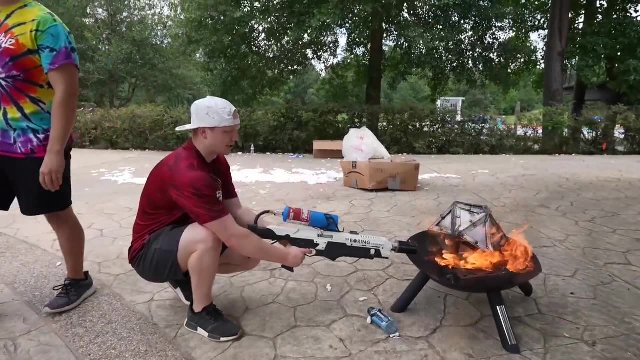 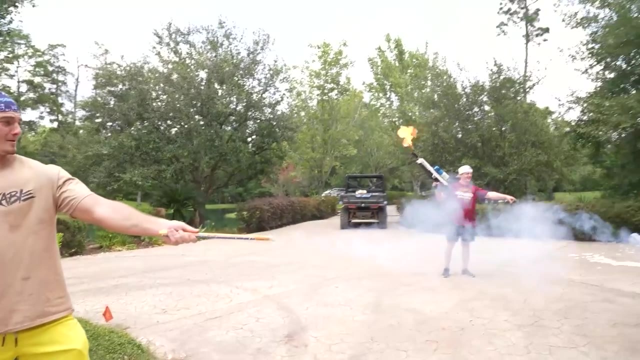 it burns. that's about it. is that max power? there we go. that is max power, there we go. we're just engulfing this boy. oh yo, it's actually working. yeah, it is, it's actually working. part of it is melting right there. chill, i got this. chill. well, i want to be a part of this. oh, hit it, you're missing. 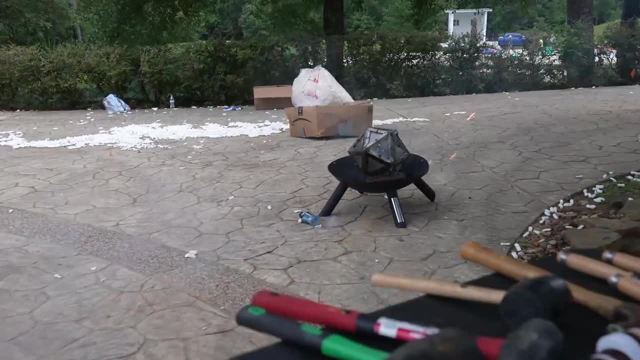 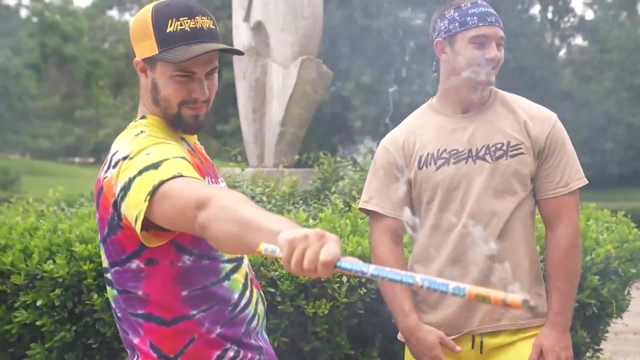 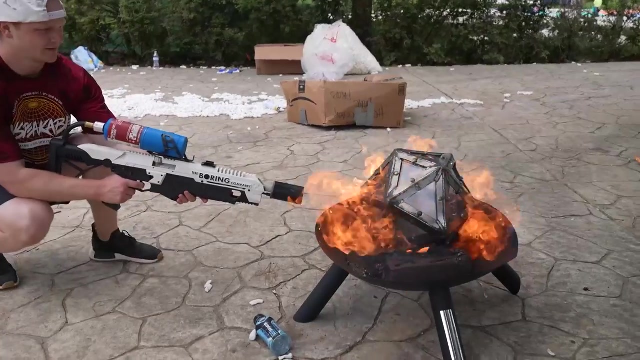 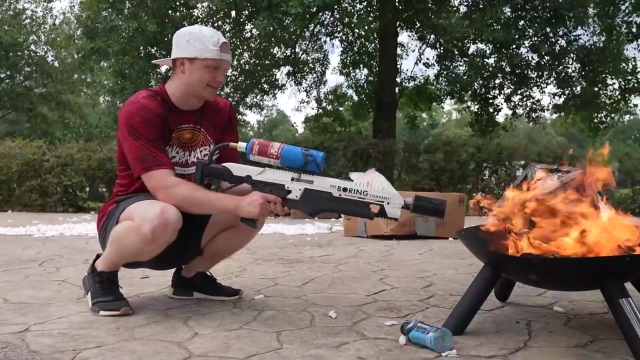 nice, oh, that's cool. hey, the last one. i think that's it. hit with the flamethrower. oh, you see that big fireball. all right, this is actually working. believe it or not, it's actually melting the glass, it just happened. open, oh nice. open, oh open. that was a direct hit. 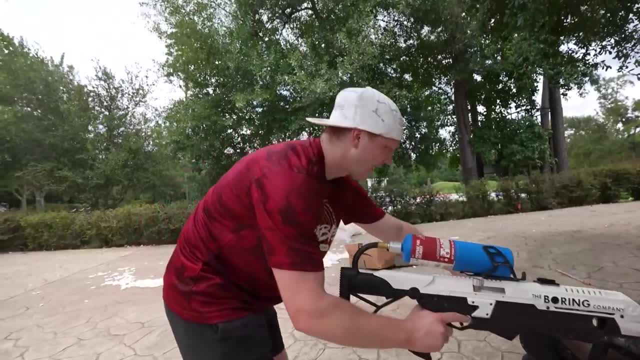 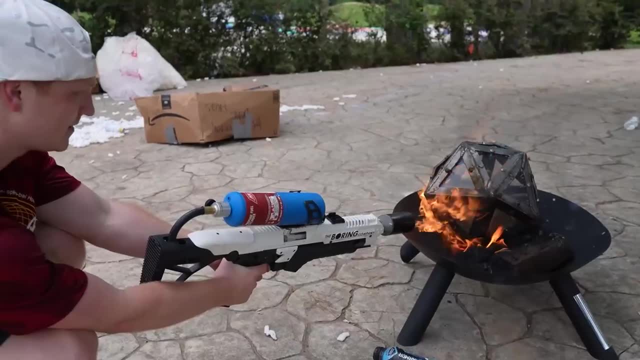 i think it's empty. let's go look at the glass right there. it's completely melting. the cube is turning a completely different color. guys, i think this is actually working. melt it right through there. fire, bro, come on, yo, i saw fire. i had to distinguish it, but it was working, so let's come check out. 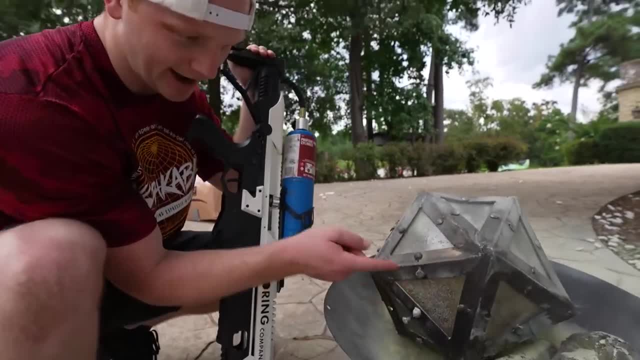 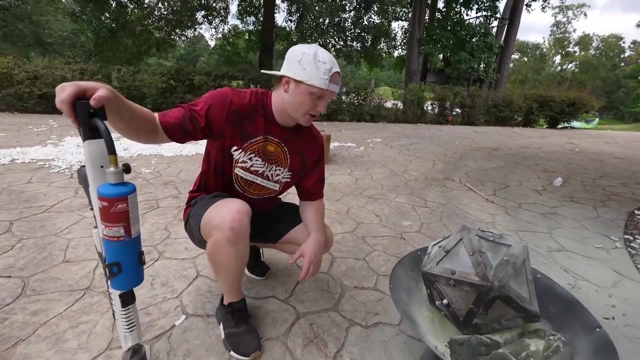 the damage. here this. i'm not going to touch it because it's very warm, but here i'll cool it down. this polycarbonate right here is actually melting. it kind of warped in a little bit. so i think let's bring a sledgehammer over here and try to hit it. it's. 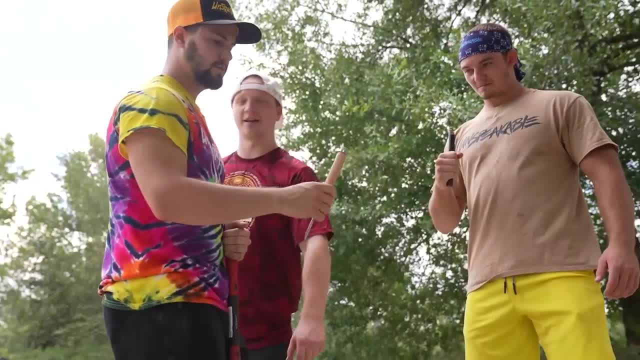 probably pretty weak right now. its shields are down, bro. it doesn't have any shields. we're gonna hit it. you wanna hold this? why you hit with that? yeah, no, if i have two hands i'll be more accurate. I'm not going to hit it hard. 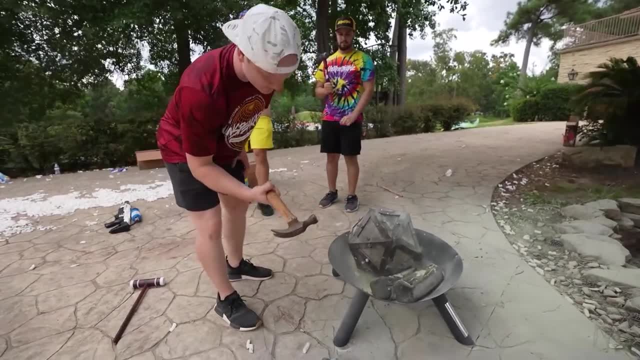 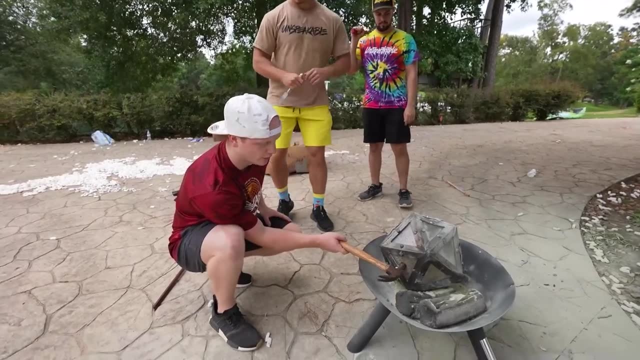 You hold it. by the way, I'm not going to hit it hard. Wait, use the other side, you dingus. Oh right, Is it starting to break? Dude, it's weak. Look, Look, how much it moves. 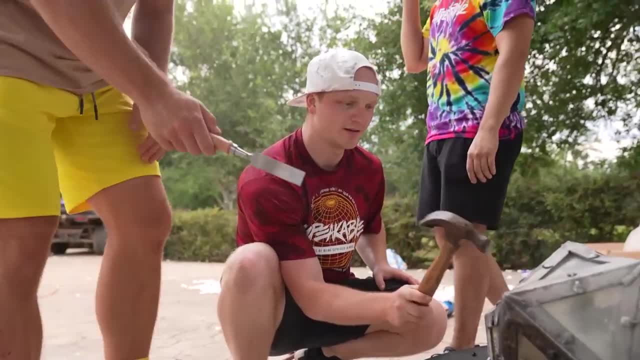 Ready. Oh snap, That's kind of flex right there, bro. Yeah, it's kind of jello-y. I'm pretty deep right there. Yeah, it's kind of jello-y because of how hot it is. Give it a little tap to stay in. 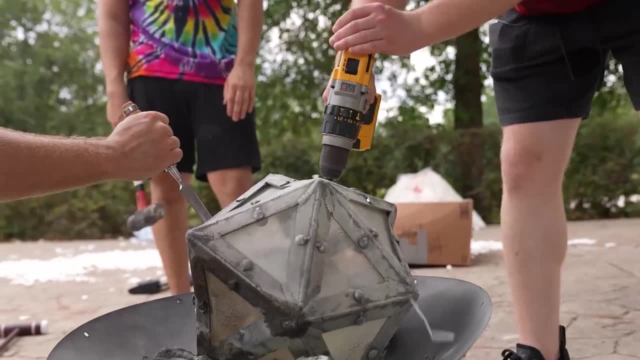 Nah, it's not going to work. Okay, Oh, he's got it. Yo, why didn't we think of this before? I don't know, That's a great idea. Yeah, you're going to have to make a hole. 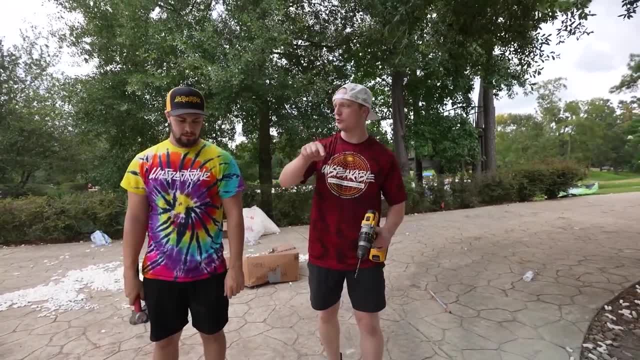 I mean, that's a solid hole right there. This is what we do. I'm going to make like four holes. Okay, I want you to hit it. It's going to make it weak. You should be able to bust right through it. 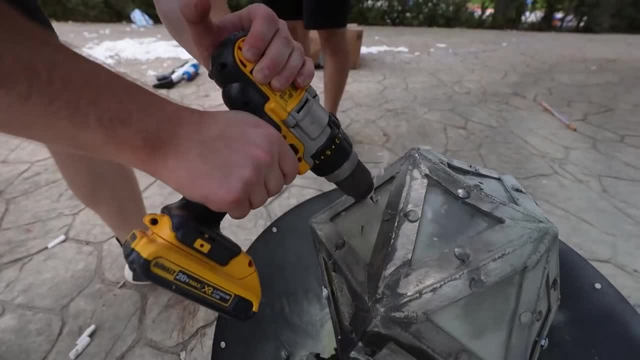 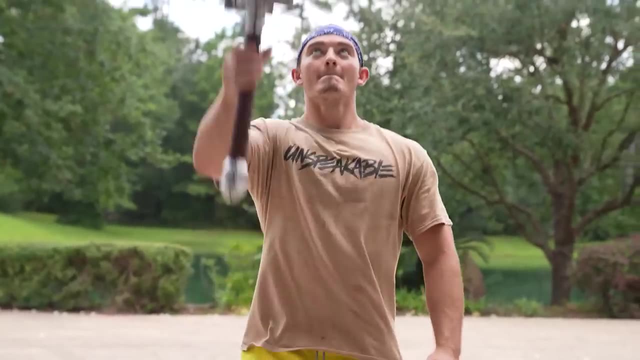 Okay, It's rubber. All right, here we go. All right, there's one hole, Hammer, I'm Thor. There's a second hole. All right, let's go on the first hole. Yo, hurry up, You're taking forever. 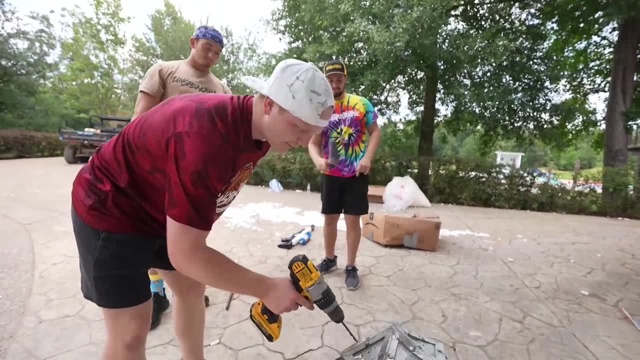 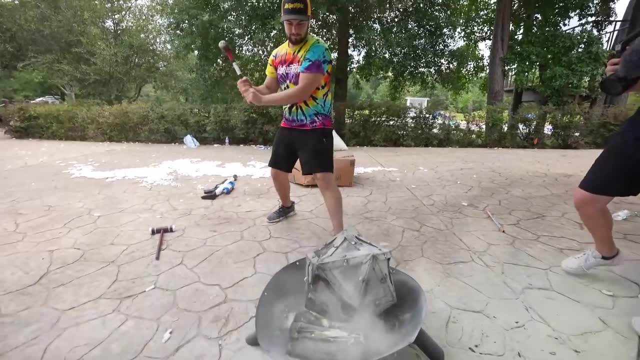 Oh hey, What are you doing? So we got a bunch of holes right there. If you can get right there, it's really weak. Go for it, Gabe. You got it. Oh, Oh, Oh Oh. 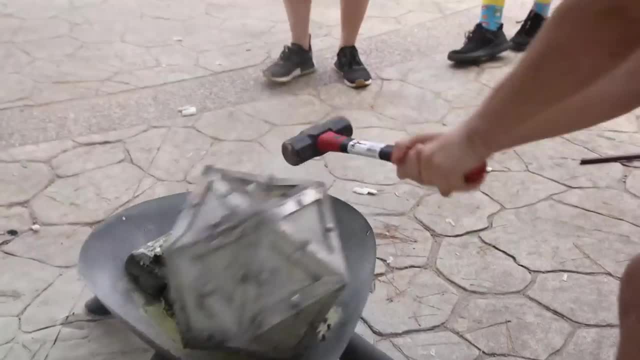 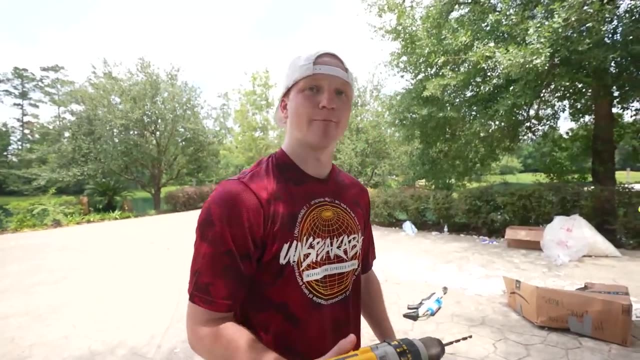 Oh, I got it. Wait, wait, wait, wait, You got it. You broke in. That's some damage. There you go. Look at that, We are in A little bit. We need to cut this metal because we can't get the money out. 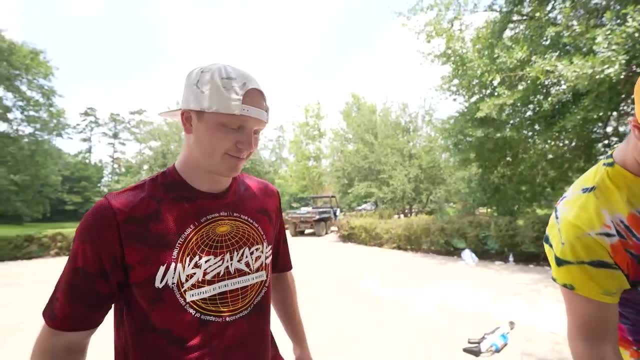 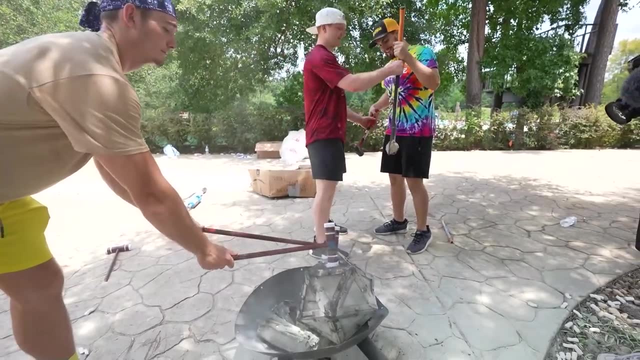 It's too big to fit through these triangles. This is a lot harder than I thought. Hey, hey, hey, hey, hey, hey, hey, I know what you need. What Cool up, Chris? Oh, hey, thank you. 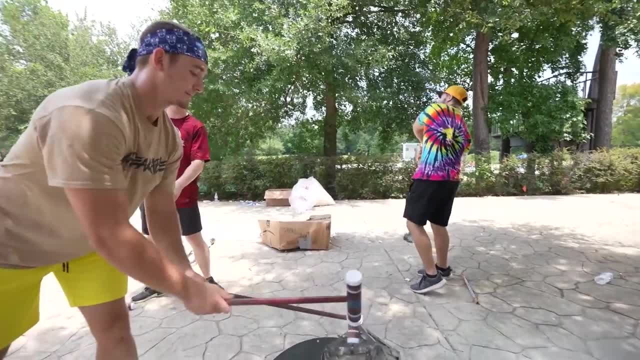 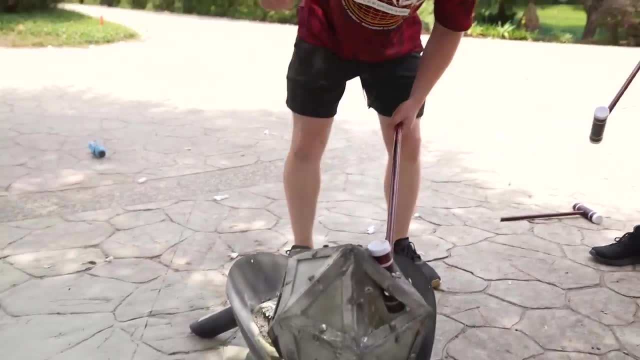 I haven't needed this for a while. Yeah, now you got a big one. There you go, You sure. Yeah, there you go. Okay, Oh Hit, Oh, Oh Wait. no way That worked And it's in. 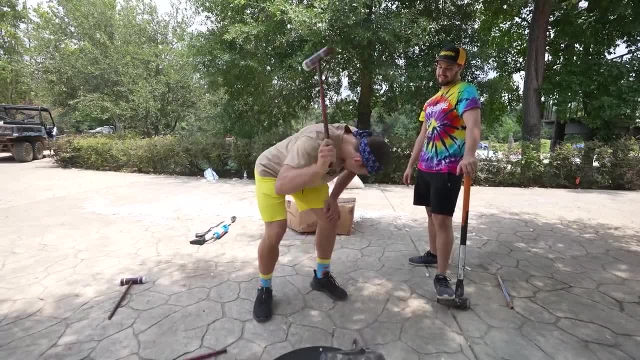 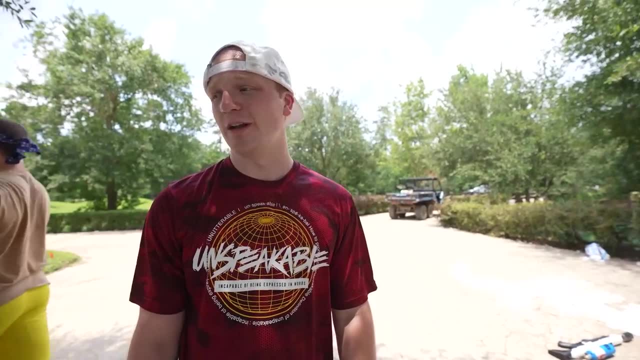 I think we just created another obstacle to break through. I'll get through. I'll get through. Honestly, guys, I think if we just hit it a lot, A lot, a lot, Yeah, Maybe if we can hit it like 40 times. 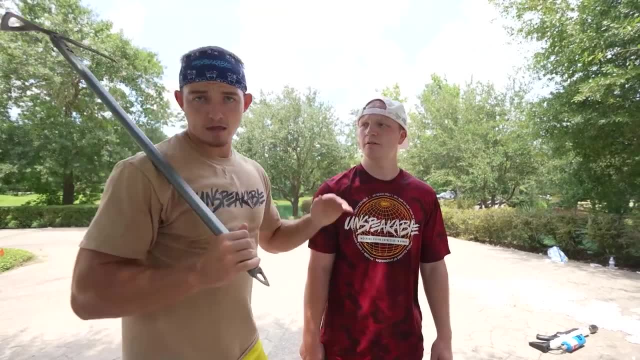 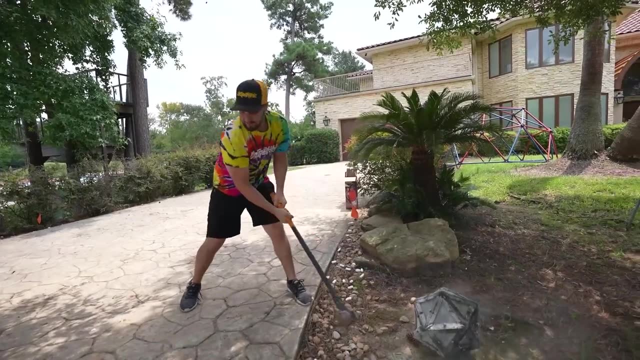 Wait, are you suggesting we have a hit montage? Yeah, Let's do it. Begin, Not gonna lie, this thing is a lot stronger than I thought. it would be All right, give it a go. This is like a 20-pound sledgehammer. 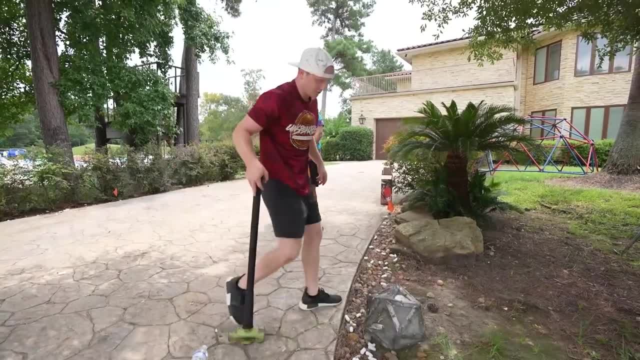 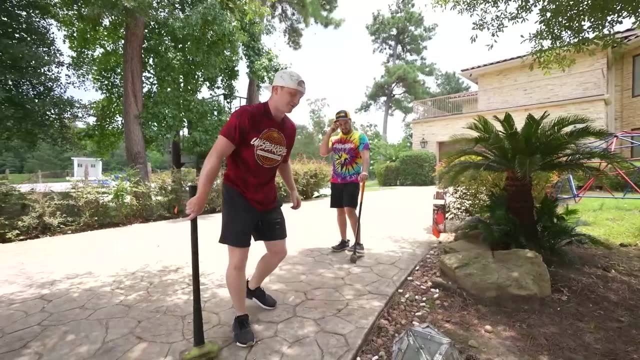 Let's get to it. Dude, I'm not even doing anything. That's how I felt. I'm literally swinging this thing as hard as I can. boys, I am not doing much damage. James, go for it, Take a hit. 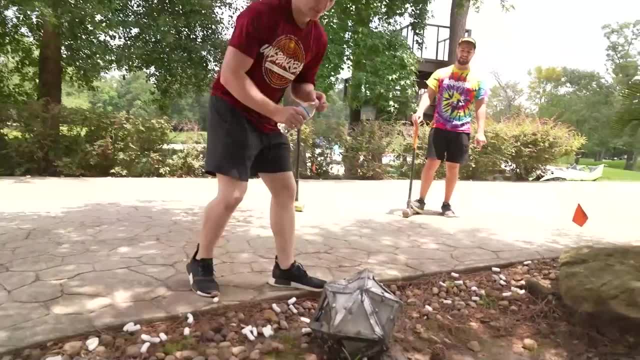 All right, your turn. What even is that thing? Hold on, Let me watch. Let me watch it off a little bit. Yeah, it's a little dirty. There we go. I think I just needed a bath. Yeah, It should open now. 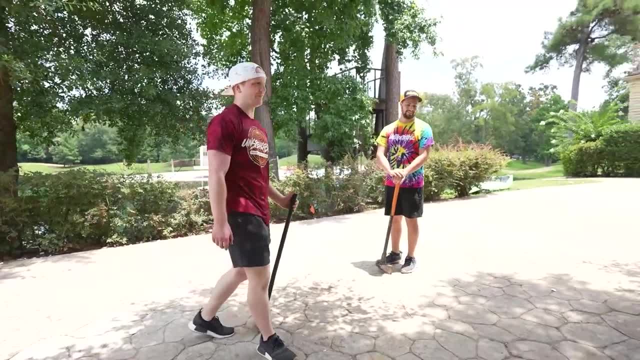 What's gonna break first, the tool or the key? Yeah, it ain't doing anything. Do you want to try the big one Here? let's get it on that weaker side. Good luck, my friend. What happened? Go the other way. 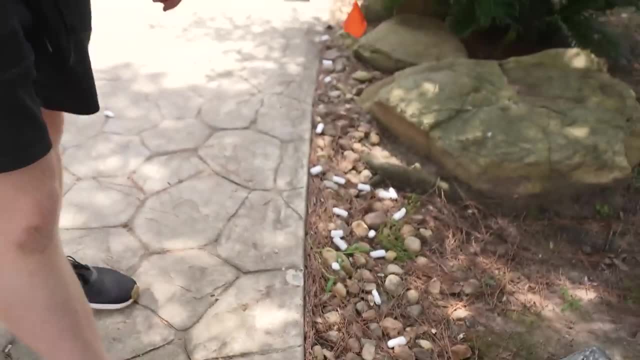 It's okay, It just broke some concrete, that's all. It broke some concrete right there. Pour some water on it, It'll be good. Oh yeah, Right, right, right right, Wait, wait, wait, wait. 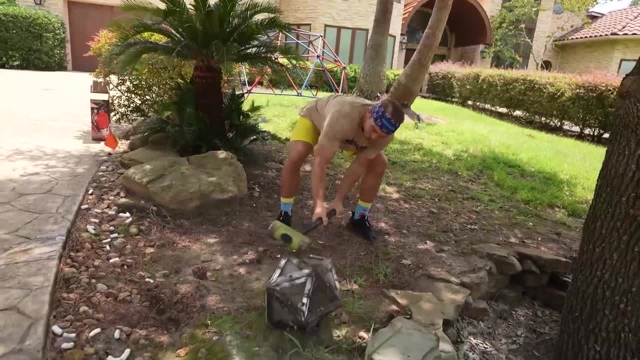 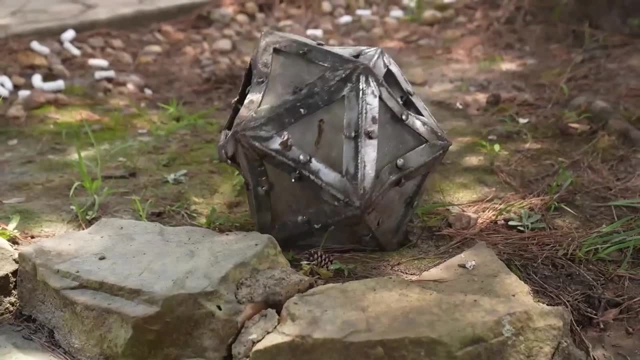 Water break. Oh yeah, See, it's good. Okay, keep going. It's fixed, The concrete's fixed. So, uh, I don't really know what our plan is to break into this thing, but I did tell you guys that we're gonna break into it, whether it takes three hours or four days. 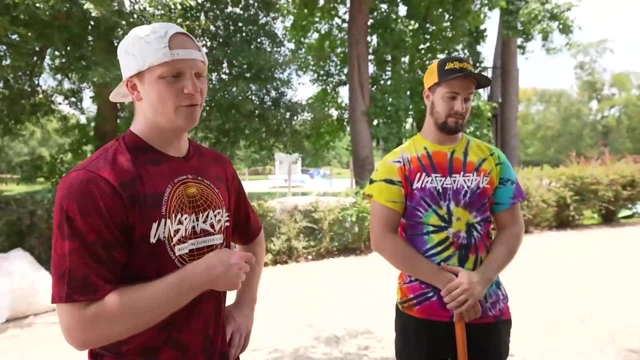 So we will get into this thing. I don't know if we leave James at it for a good while, If we give James some good energy drink- Oh wait, Look, look, A bunch of water. I think it's breaking. 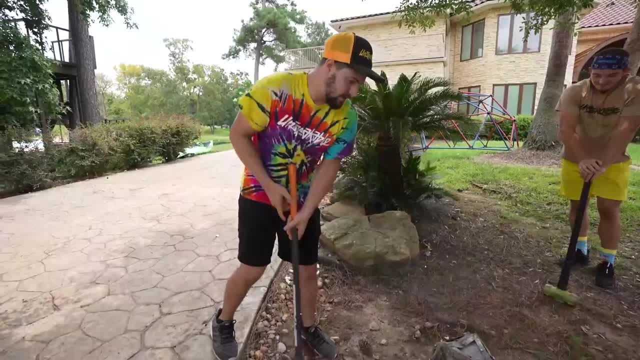 It's breaking. Okay, so he's dinting it really well. Damage report: All right, flip it over, flip it over. There's damage. We have been really bending this side right here. The problem is is we need to like bend this steel? 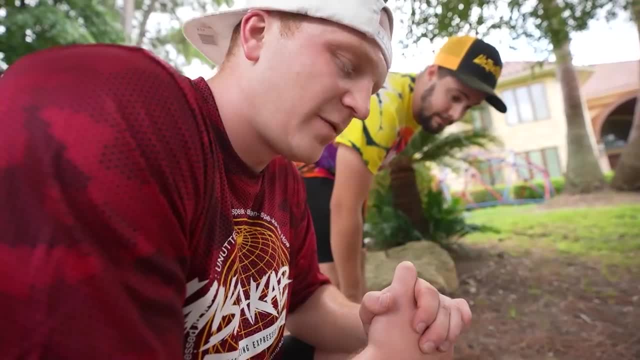 Oh look, It ripped it. It'd be really nice to have the jaws of life. That would be great. Fortunately, we didn't have that. I'm sorry. You know, if we just keep swinging at it and don't give up, our dreams can become dreams. 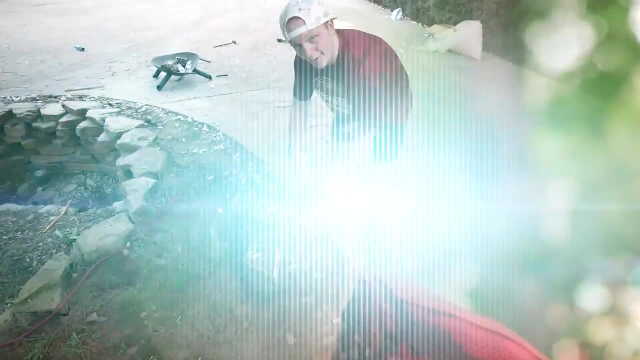 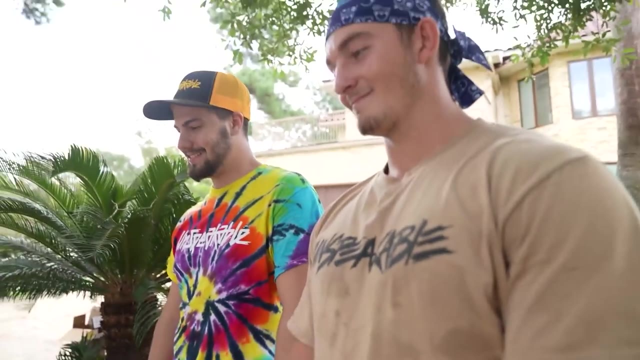 Yeah, I like that. Our dreams will become dreams, True dreams, Reality. All right, boys, This time power tools, We're going in. Yeah, I feel like Bob the Builder. It's working, Look at that. All right, I'm going back in. 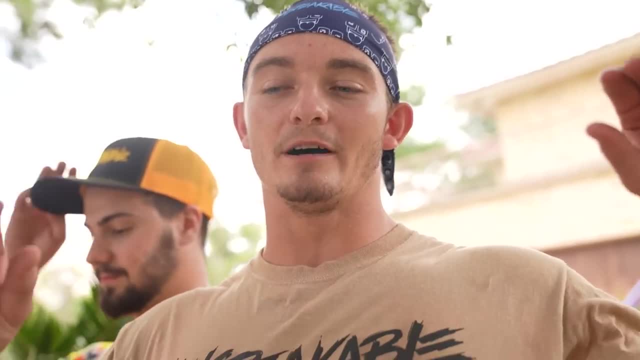 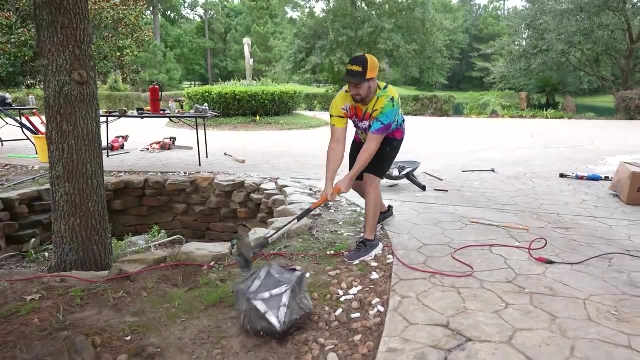 Yo, someone put a side-by-side of Gabe in the excavator from Bob the Builder. Hey, give it a hit. Hey, hit it right here. I'll try my best. Hold on, Let me go back in. I'm completely through. 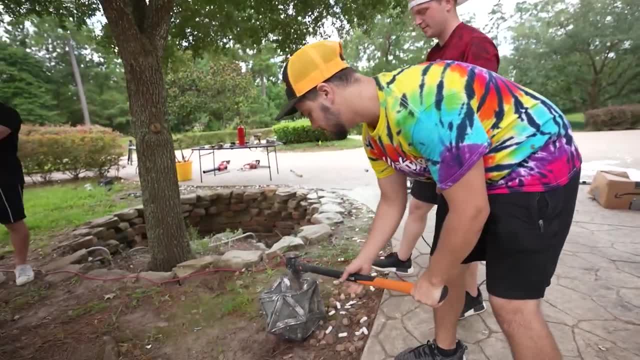 Look at that, It's a clean cut right there. James, I got an idea. Can you come and give me a good swing, Not like super hard, but yeah, give it a good swing. I don't know. 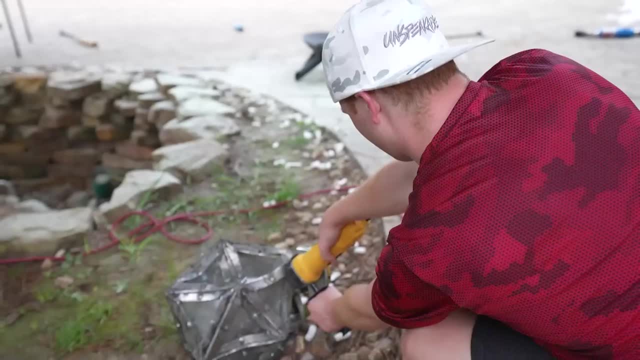 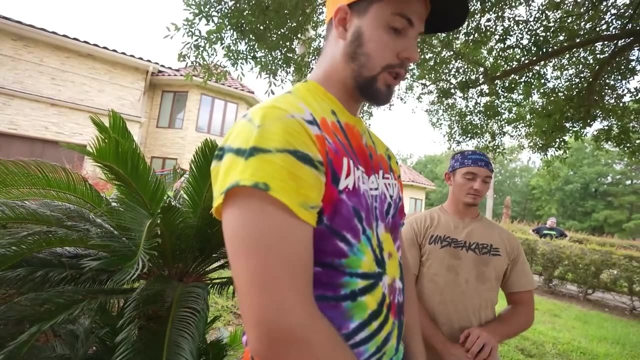 Oh, look at it, Is it going to work? No, that worked, Did it really? It broke it apart a little bit. yeah, You're almost there. Keep going, Almost there. Keep it going, You're close, Oh fuck. 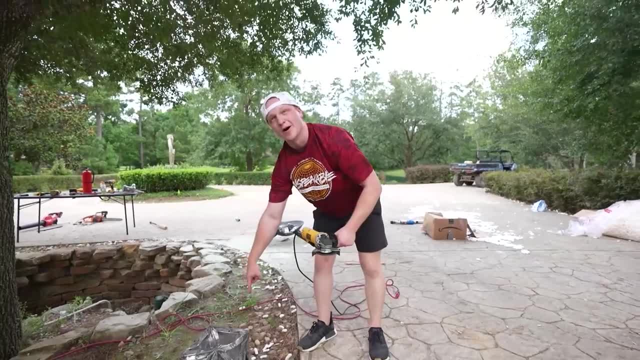 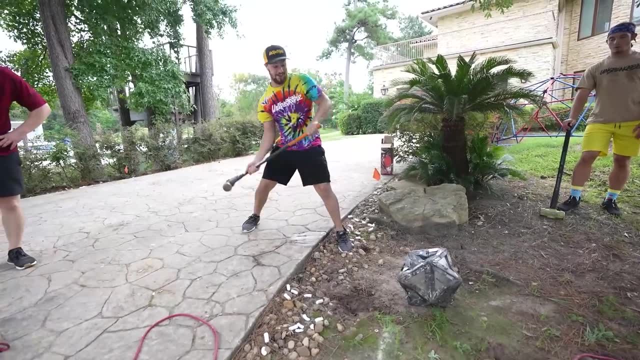 Super close. Such a good job. All right, If you guys can hit it Right there, I think we can bust that entire part off. Did I miss it? Yeah, you missed all of it. Oh There it is. There it is. 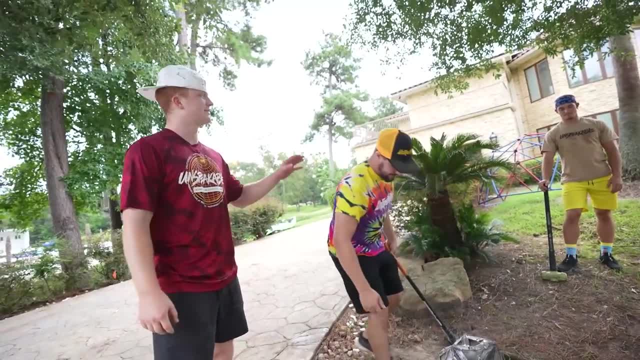 We were so close to making it. How is this not falling off yet? Yo guys, All right, real quick. Which one do you think was harder, the unbreakable box or the unbreakable cube? I don't know yet. 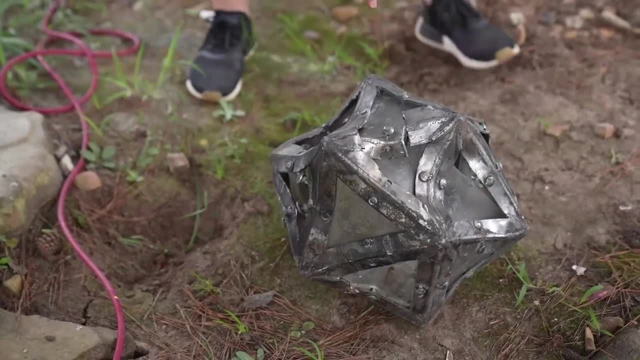 We're not done. Smack, Oh, Oh, my God. Oh that boy Off off. There was a little piece hanging on. It's the bolt. Yeah, Oh, the bolt's holding it on. You probably cut the bolt off. 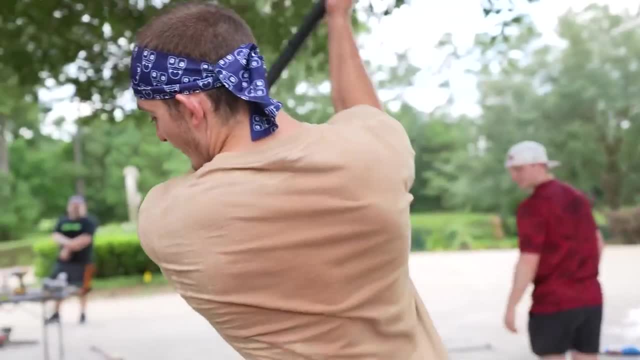 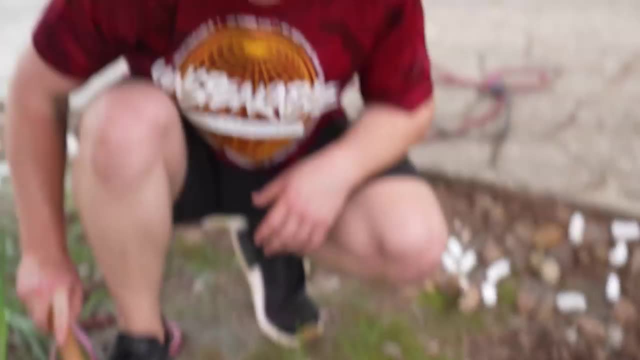 Oh, I think we can pry it off. Why pry it off When you have a sledgehammer? Smack it off. Yo yo yo Hey, Look at that. I'm not going to touch this piece of metal because it's insanely hot, but, as you can, 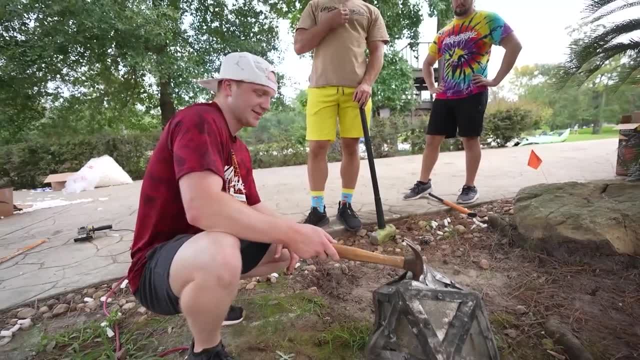 see, that is off. Now we just need to get through this. Honestly, dude, if you hit this, it would break The metal's the hardest part. Give it a nice smack. Oh, there you go. Hey, look at that. 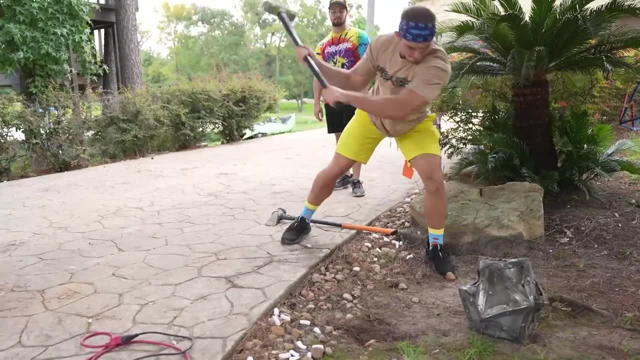 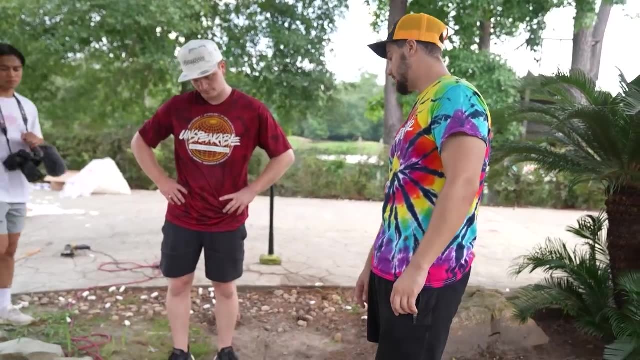 Look at it, You bent that metal really nice. I like that. Keep going, bro. Okay, so we cut this piece off. We dented the whole thing. I mean, cutting This thing will eventually work. Woo, Right now we're cutting all the bolts off. 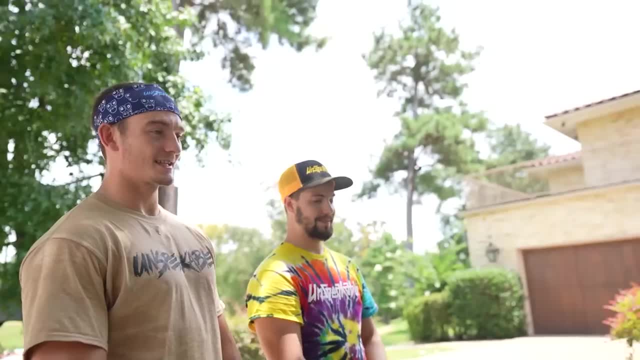 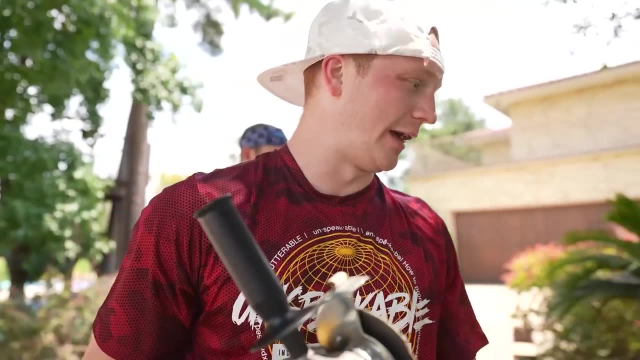 Give me that next one. All right boys. So I'm sweating. This thing is done. As you can see, the blade there is completely gone. So this thing is out of the mix, but we cut off a lot of bolts. 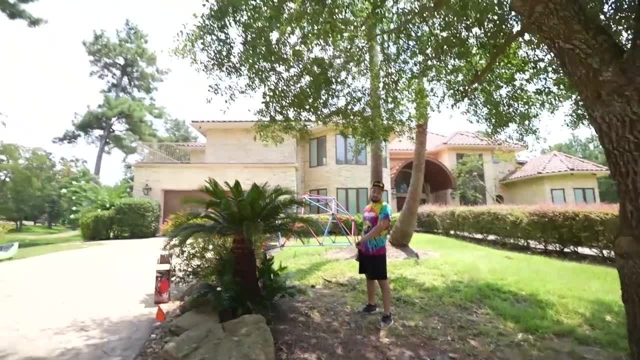 So hopefully we should be able to take some swings at it, Break it a little more. All right, James, I guess we're just going to keep smacking it till it breaks. Just smack it, Just go, Smack it. 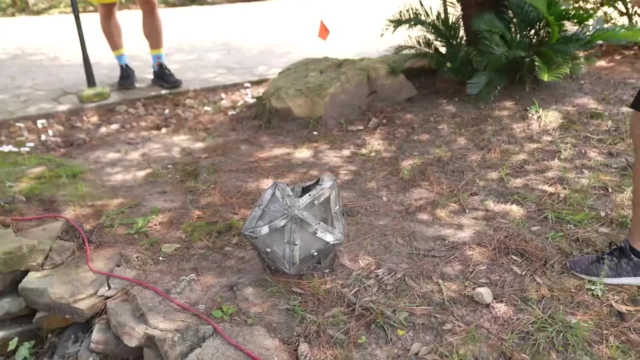 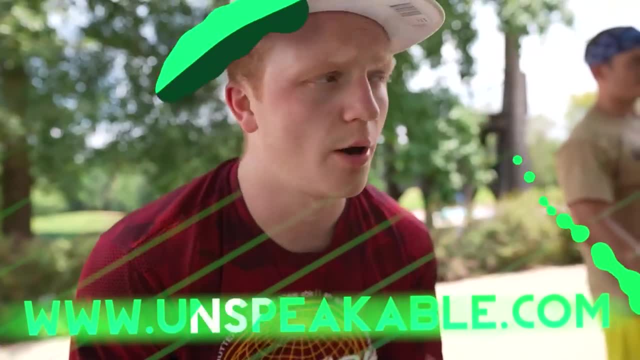 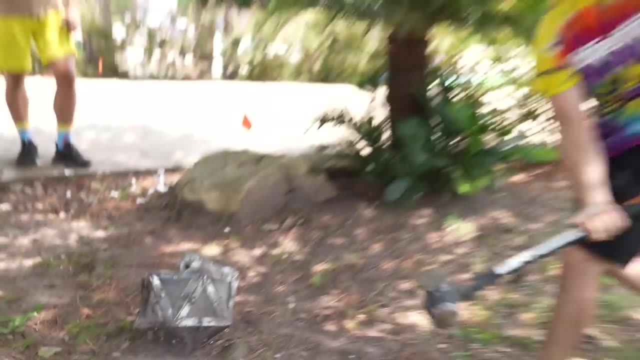 Give me that merch power. Guys, go to wwwspeakablecom, Get your merch. We got brand new shirts, Brand new hats. Merch power, Let's go. Merch power, Let's go, Let's go, Merch power. 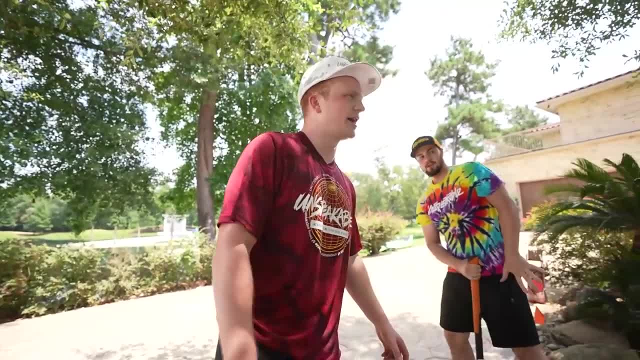 I got to recharge my merch power. You want to give it a good smack? Give me a scream, James. Give me a scream. I'm going to get hyped. I don't like scream, bro. You don't scream, No. 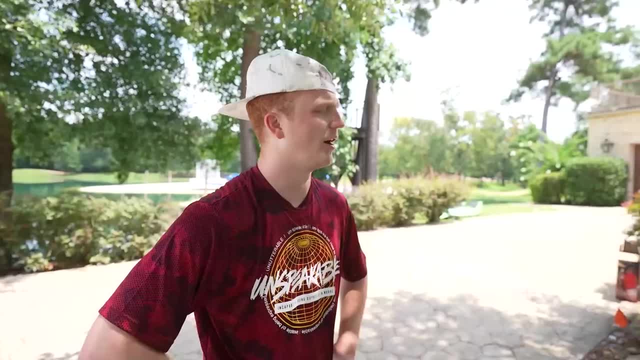 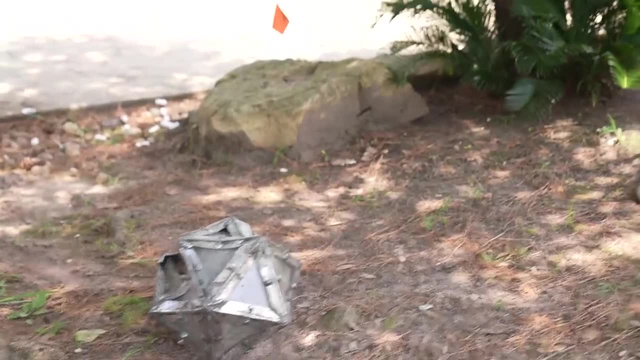 But, like when someone scares me, I go: hello there, Do you yell? I'm going to hit the cue. All right, hit the cue, bro. You got this Merch power baby. What's that? There's the scream I was looking for. 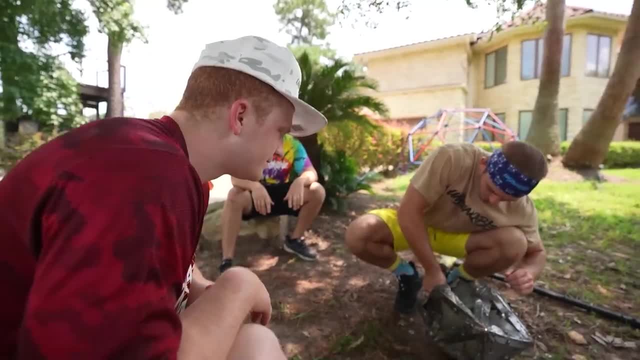 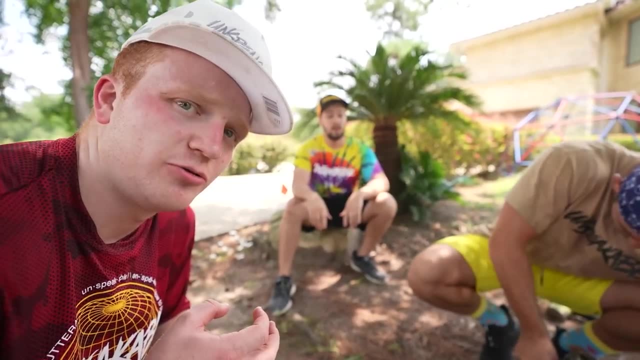 What's the problem, James? My calculations of aquatic animals. it's these little sheets of triangles right here, These little carbonate things. They're all conjoining together. The problem is, is we're actually making the cube stronger? You know, I think the way Dustin designed this thing is: when you hit it, it forces everything. 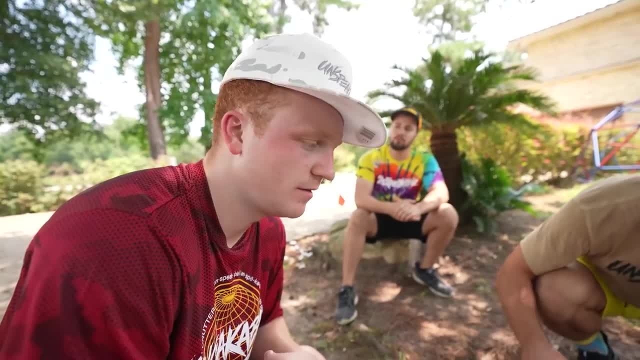 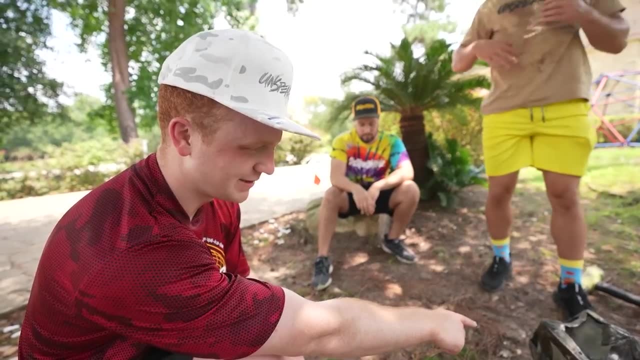 together, wedges it together, which actually makes it stronger. Very troll-like, Because right now this bolt- you can see right here, yes, is going into this one. If we don't get some of these big plastic pieces out, we're actually making the cube stronger. 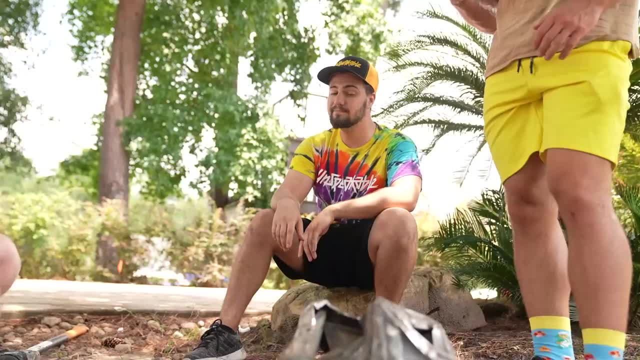 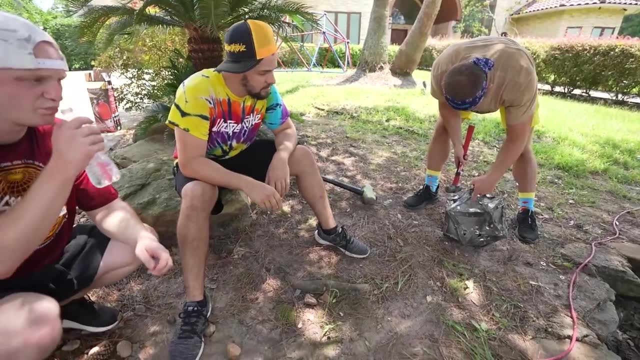 Maybe it needs another massage day. I think it does need another massage day. Do you think so, Honestly? I think I need a massage day. It's probably stressed out. Yes, I mean, Oh, you did something. I broke from this triangle to this triangle, to this triangle, to this triangle. 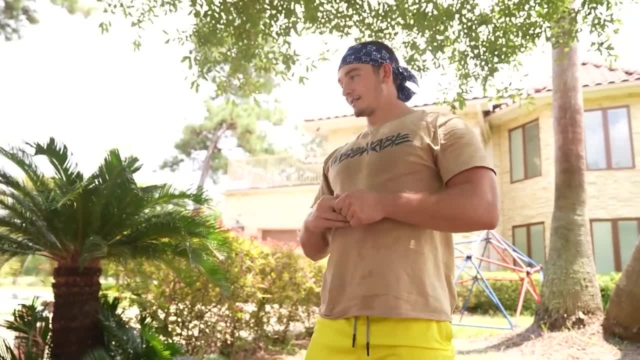 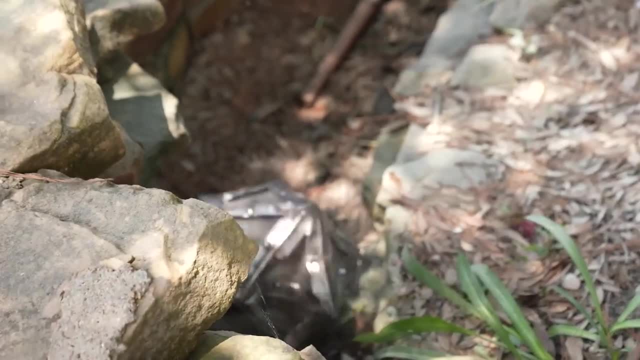 So if we could basically pry and work around the bolts and nuts, we could get in. We're going to do this today, guys, Before sun goes down. we are going to do this Honestly. Could we just leave it there and forget about it? 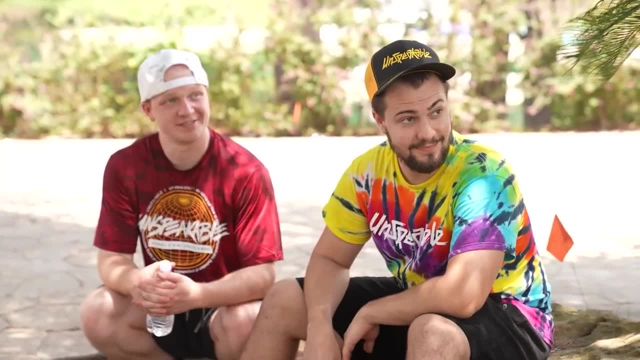 Yeah, I don't like that. I don't like that idea. Tubing: You want to tube Jet skis? Who wants to tube? If you want to see some jet ski tubing action around the house, go to the speaker books. 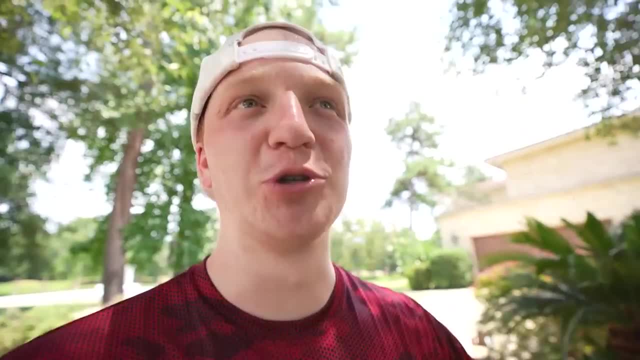 and point out That's literally all we film. The whole channel is just tubing. We're jumping the hills, It's lit, We love our tubing And we're going to do it again today. Let's smack it right there. Give it a good smack. 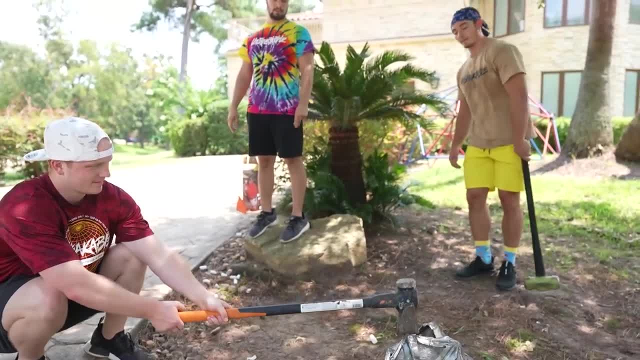 That right there is all broken. Smack it. That's not going to work, but I'll hit it. Go What. What do you mean? that won't work. It didn't work. Do it again. Do it again, Smack it. 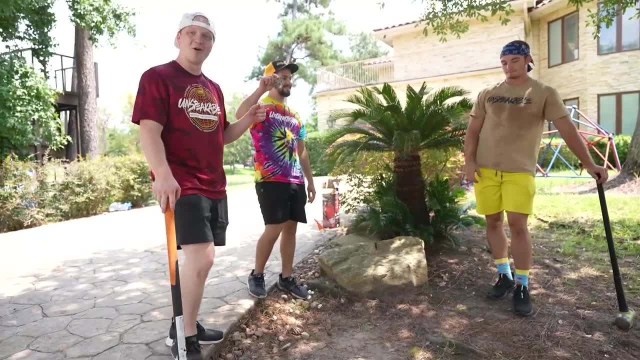 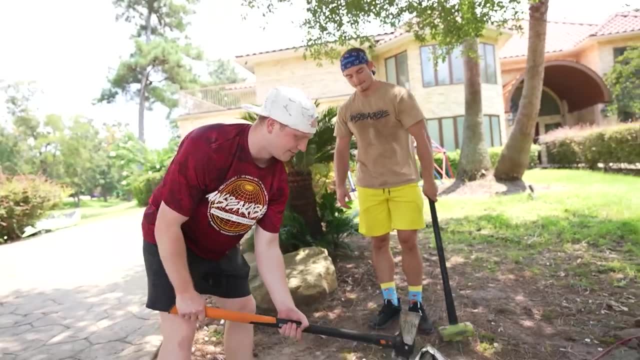 Hey, Whoa, No way, That's another piece off. Let's go Smack it. There you go, Wait, wait, wait, wait, Wait a second. Grab it. The bolts are working against us. Get that piece of metal and bend it back a little bit more. 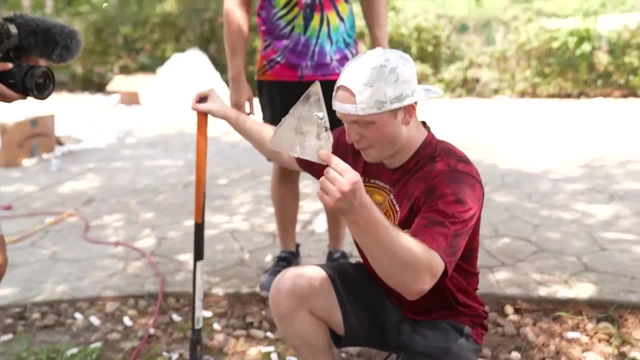 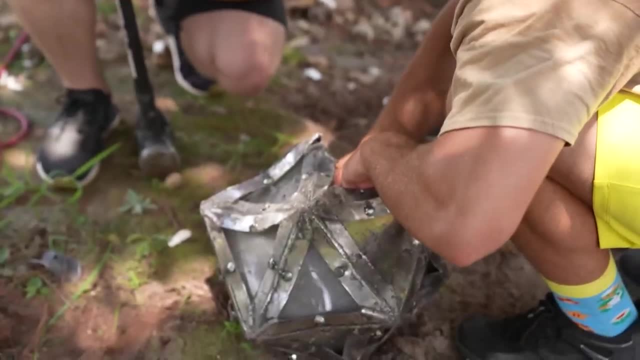 Oh, there, it is, There, it is There, it is. Are we in? Yes, One piece. One piece is out, Finania. If we can get this one piece out, we are in. It's like a big puzzle game that we don't know how to play. 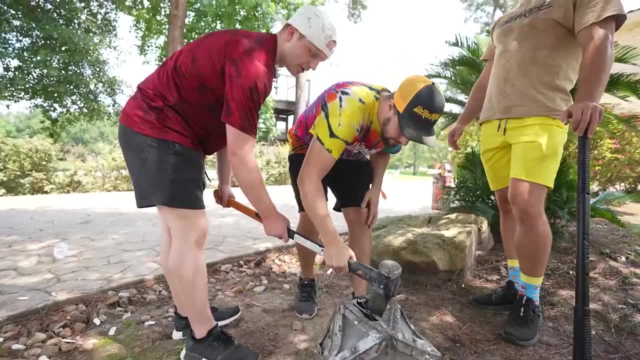 Because we don't play puzzle games. Put the X face in that way. Brett, Are you trying to knock off that bolt? You can't just unscrew it. Sorry, I can hold it. Wait, hold on, You can't just unscrew it. 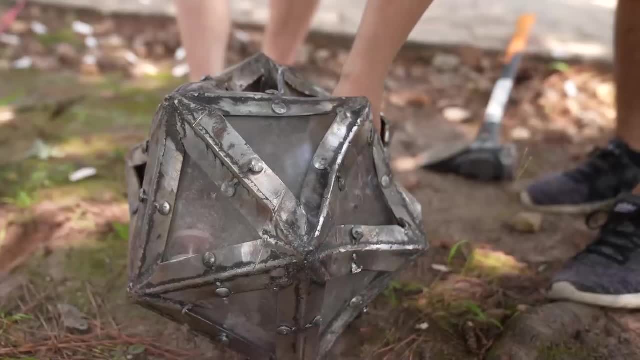 Oh yeah, I think you're right, We're on the inside. yeah, Bro, you can just unscrew it. I mean that wasn't what we were going for, but might as well. I mean we're going to hit that bolt. 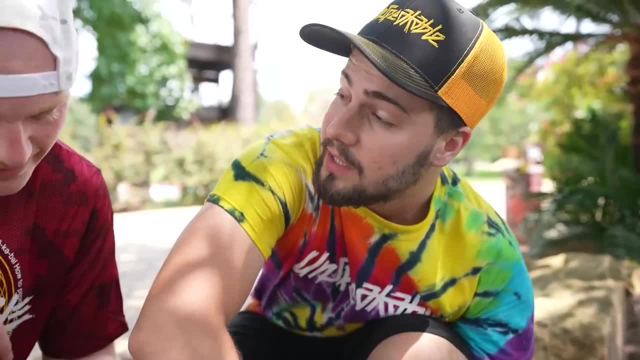 Bro, you can just unscrew it Now that you mention it. that's a good idea. It kind of got cut off. It's stuck. Yeah Yeah, the metal's all bent so it doesn't want to work. No, there it is. 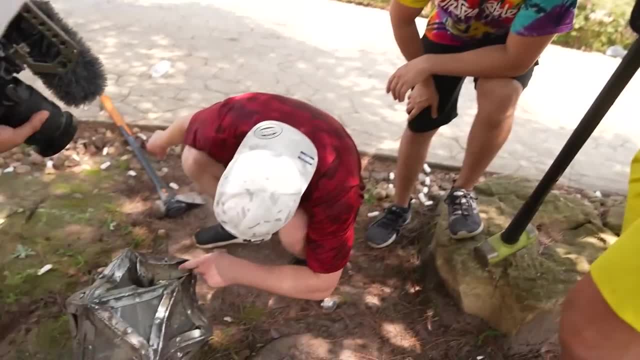 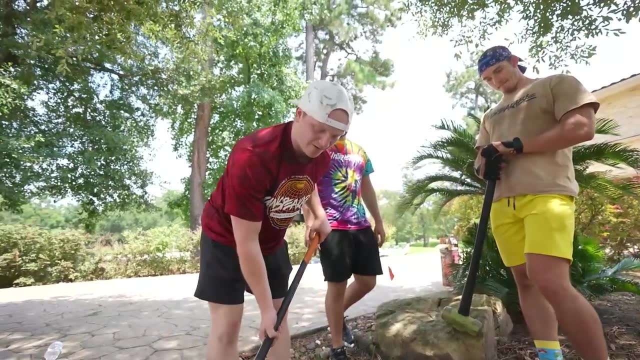 One hit, This piece is out. Where's the money? Oh my gosh, It's stuck against this piece right here. Hold on, No, it's not moving. I got something, though. Part of that hammer thing, Yo the pot. 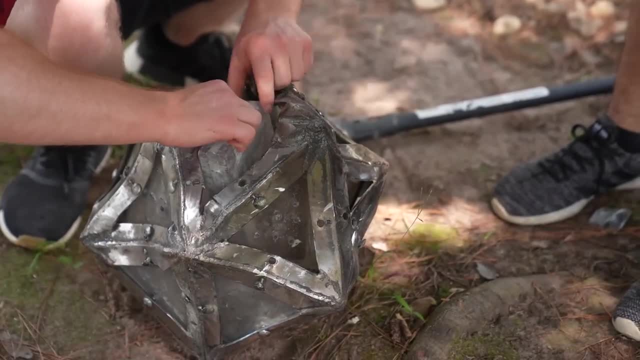 Oh wait, Oh wait, Oh, come on, You can do it. Oh, come on, You can do it. Yes, Yes, there it is. Now we have to break into this Dude. no, Bro, come on. 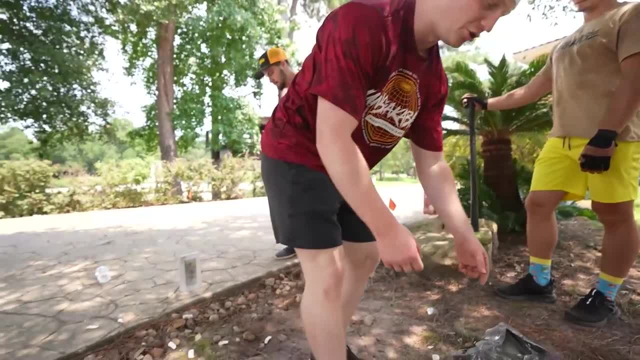 I said: just the cube, Bro, we got to get the money out of it, All right, so the cube has officially been broken into. I was hoping that would work. Yeah, we're going to need something very sharp. Yo, honestly, that might work. 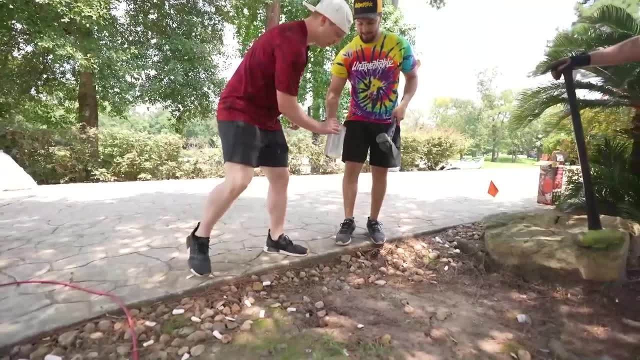 Yo, stand it back up, Put the ax part on it. Oh yes, Split it. So look, There's three layers right here We're going to try to split. Yo, wait, This part is already open. Wait, how are those layers connected?